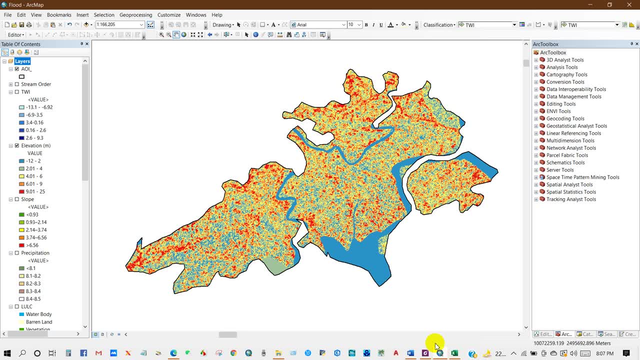 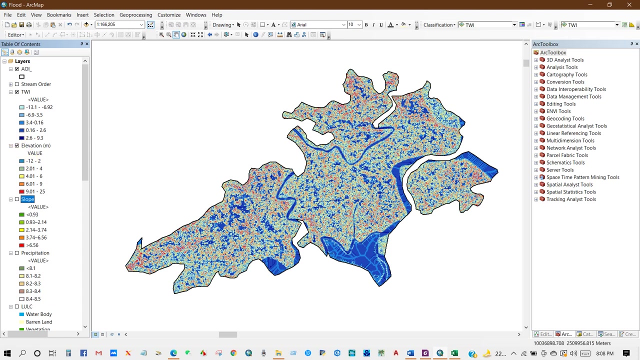 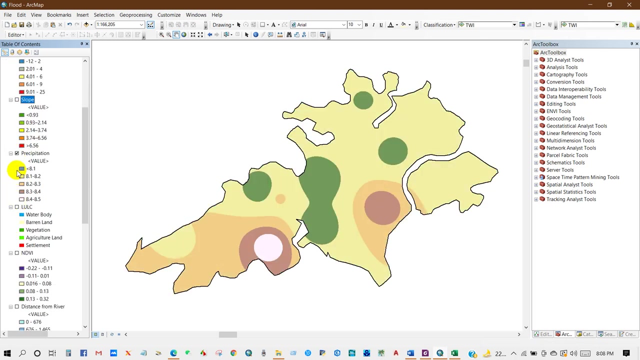 and increases the possibility of flooding. flood intensity and frequency are very high around our drainage basin area, particularly closer to rivers. high values of topographic wetness index correspond to areas favoring water accumulation and high runoff, and also in land use and land cover change dynamics. parameters affect hydrological processes. components such as infiltration, surface runoff. 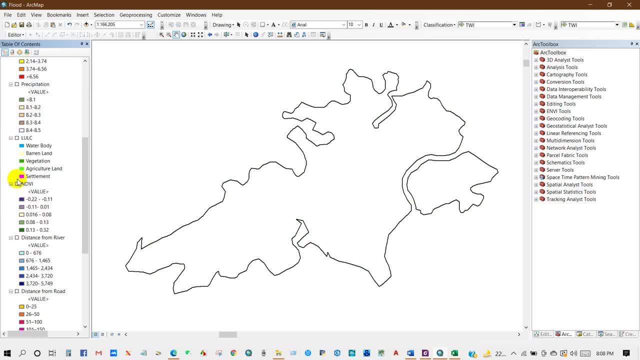 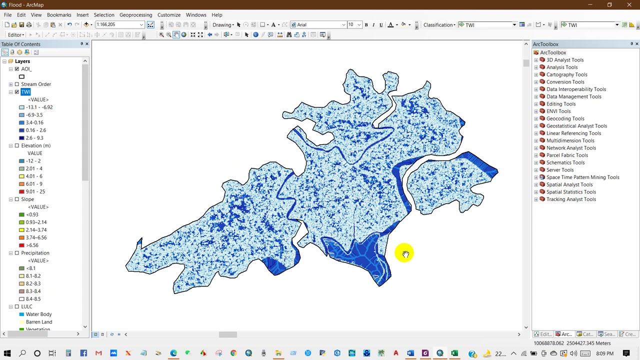 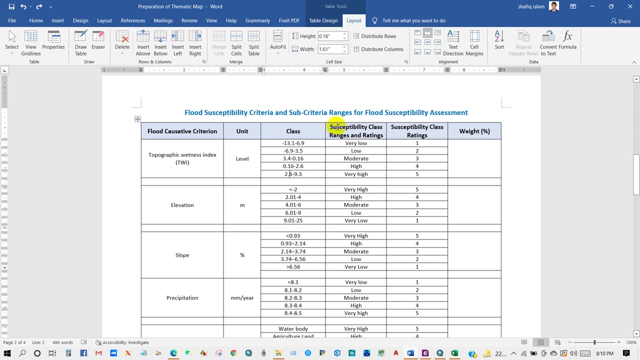 evaporation and evapotranspiration, and hydrological activities. this will be discussed with you only when learning more about the flood causative factors. in order to combine the data set, they must be in a commonly scale. we have to reclassify all the thematic maps and need to be organized on two five scale for each factor. 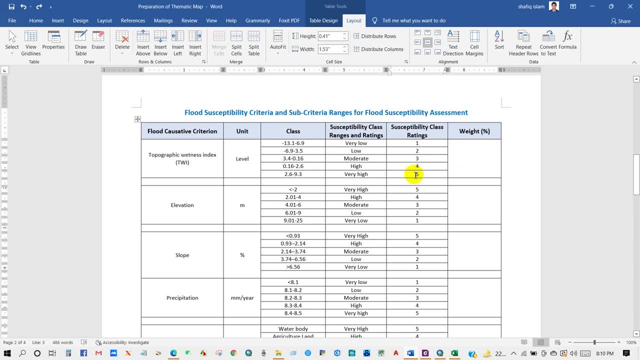 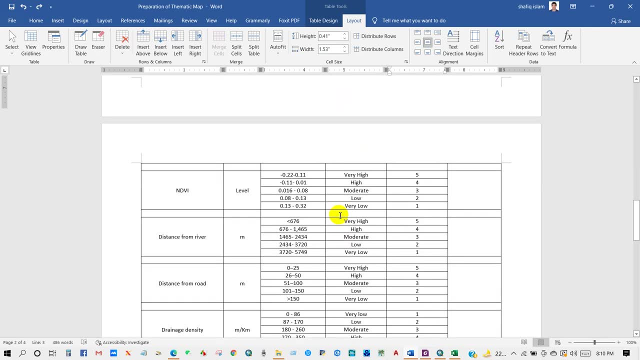 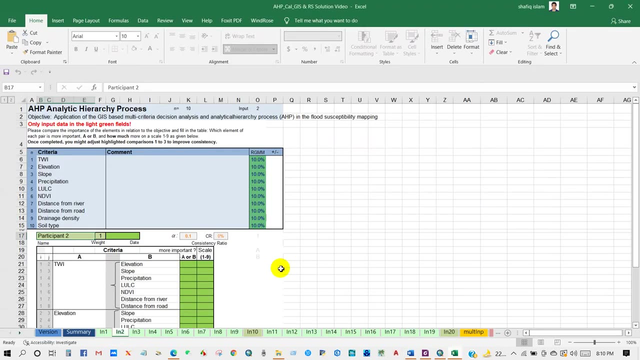 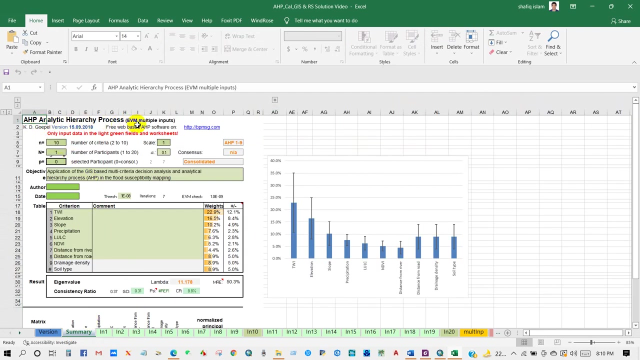 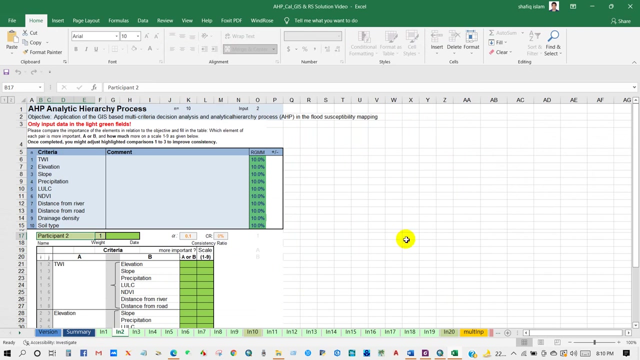 the arian for weight calculation of all factors. i will use asp techniques- multi-criteria analysis using this asp excel sheet. you will just need to your expert opinions to rank the factors and put the factors in this excel sheet and it will calculate automatically and give you. 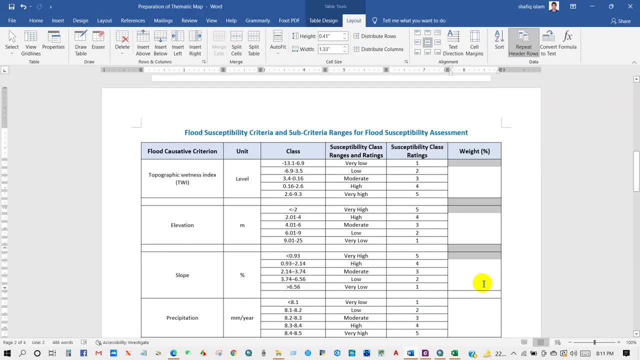 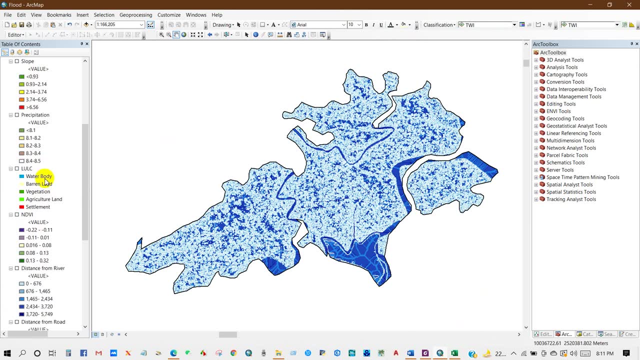 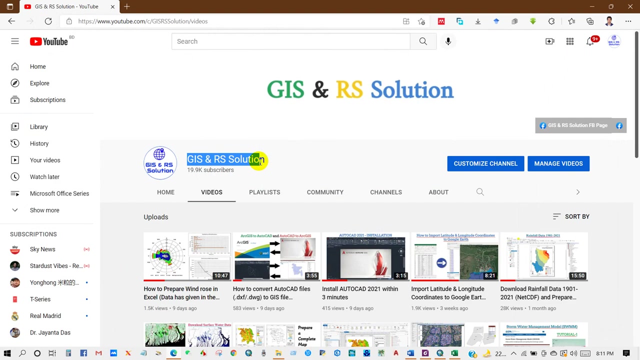 the weight. i have shared the download link of this asp excel sheet in the description section of this video. you can download easily. i did not show here most of the thematic map preparation as i have already uploaded all the thematic map preparation process in other videos in this channel. just go to my channel and click in videos. 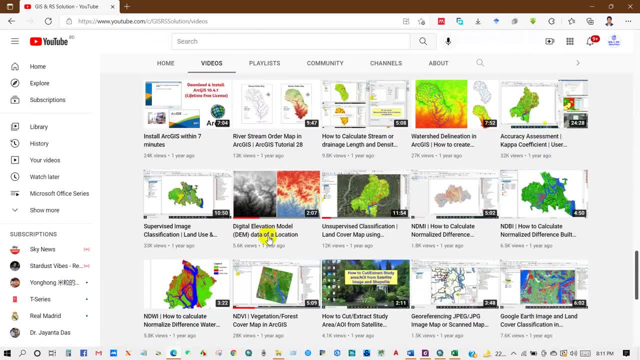 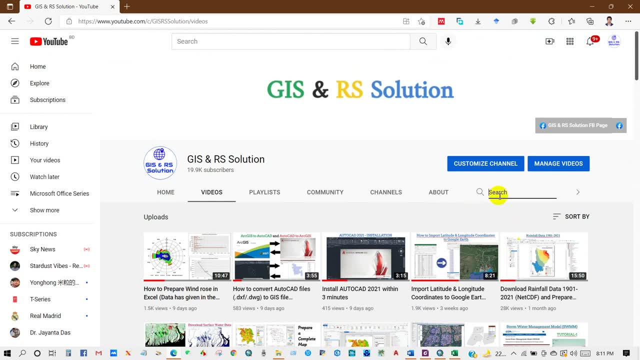 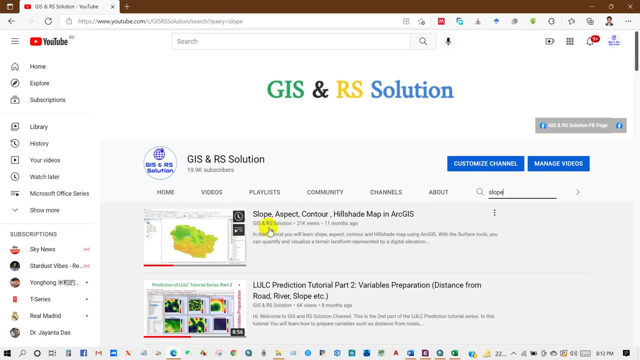 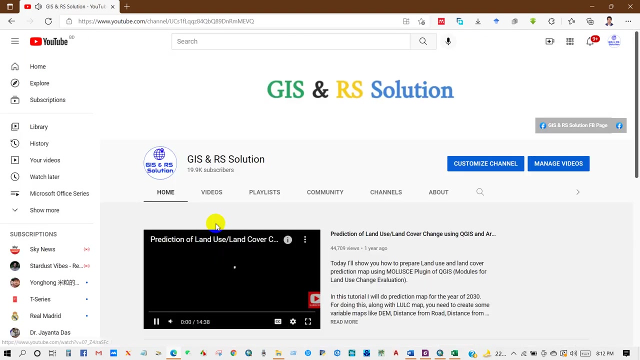 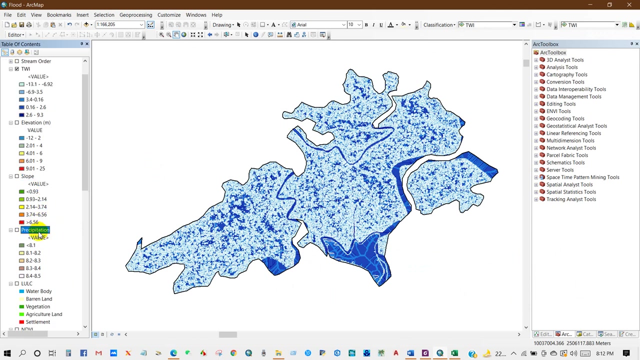 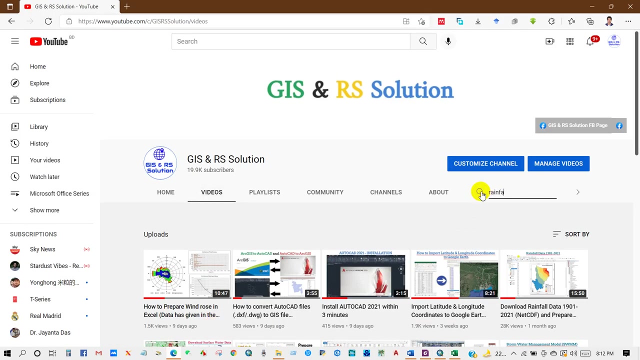 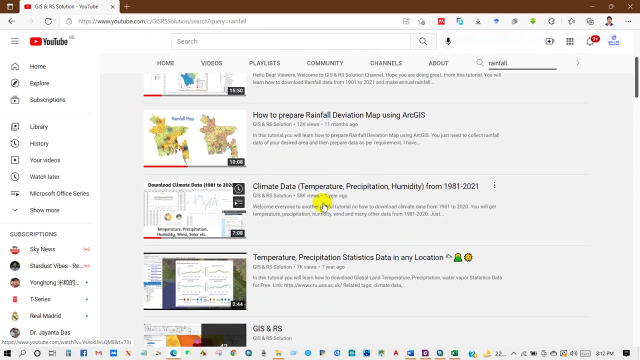 and here in search box just write slope and you will find the slope preparation map, how you can prepare a slope map. and if you want to get how to prepare precipitation or LULC or elevation, just search here like rainfall, you will get the rainfall map preparation video. from here you will find everything about. 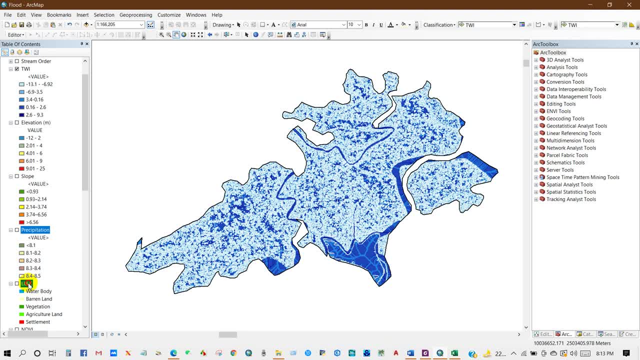 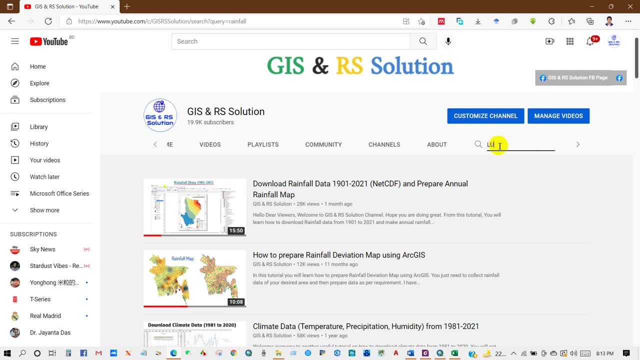 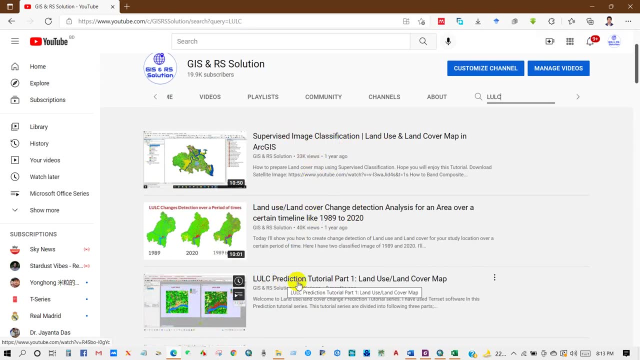 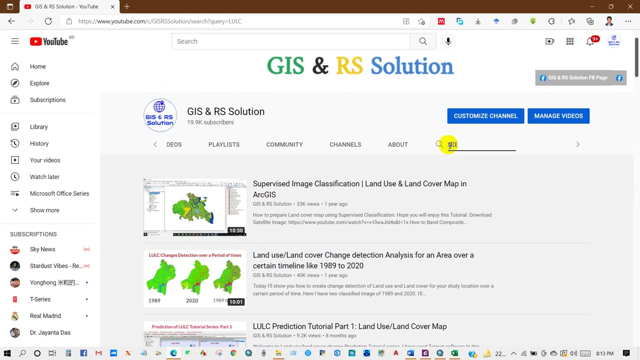 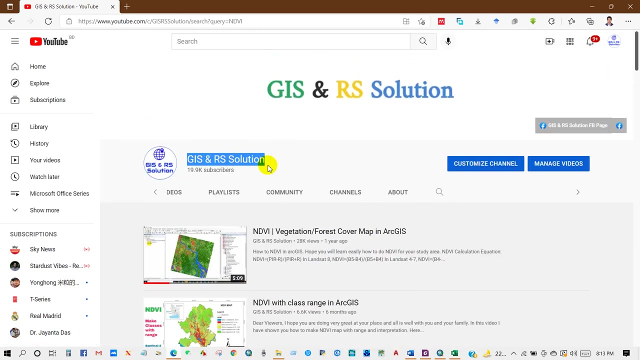 thematic map preparation from here: LULC, NDVI, everything LULC, and you will get several land use land cover map preparation technique in ArcGIS in NV, supervised, unsupervised classification technique for land use land cover map preparation. also you will get NDVI preparation. I have given the link in the description section of every thematic. 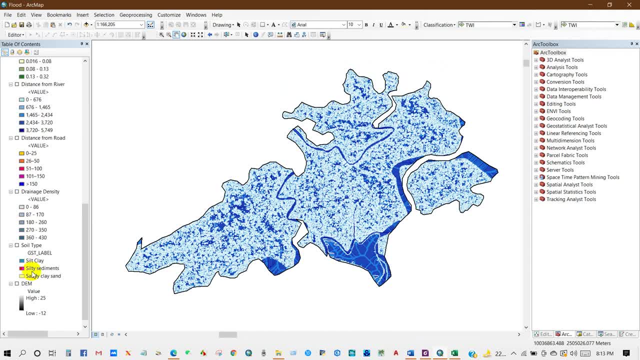 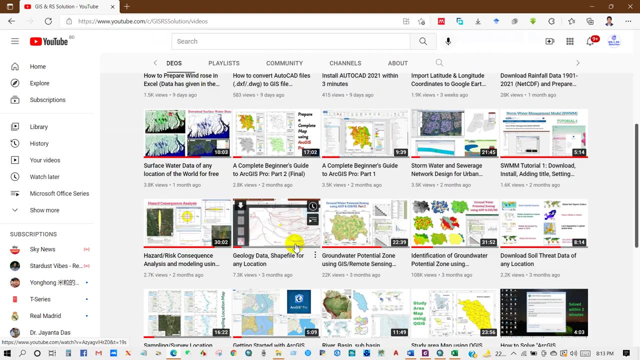 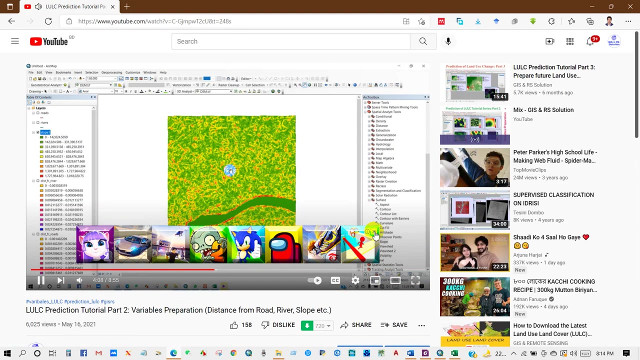 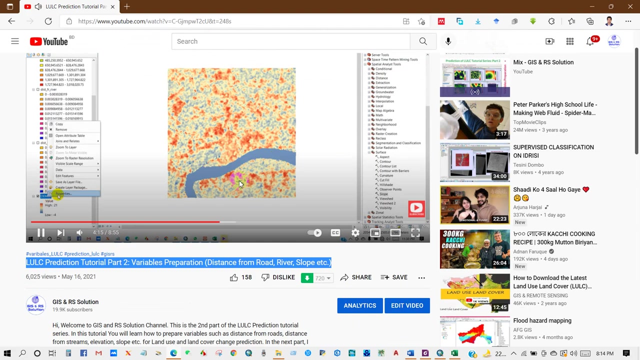 map preparation process that has been used in this video: distance from river, distance from road, drainage, density, everything. every thematic map you will get from my channel. that's why I did not show you in this specific video. in this video I have shown several variable preparation, like distance from road, river slope and others also. you will also get this thematic map. 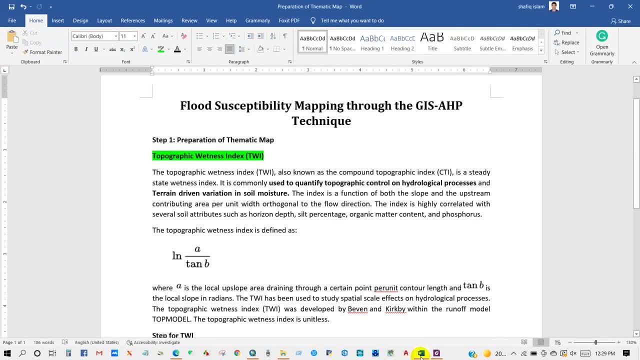 here. i did not upload topographic witness index map yet in my channel, so first i will show you how to prepare topographic witness index map. so topographic index map, it is also called compound topographic index. it is used to quantify topographic control on hydrological processes. 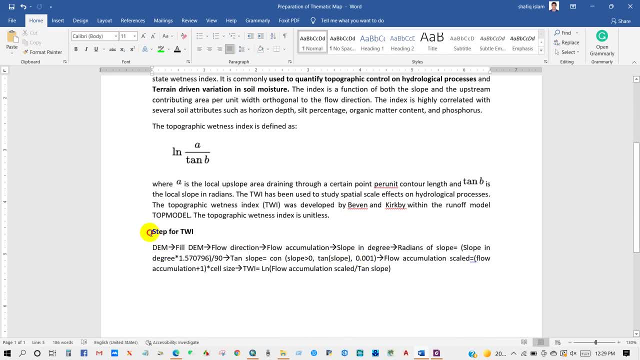 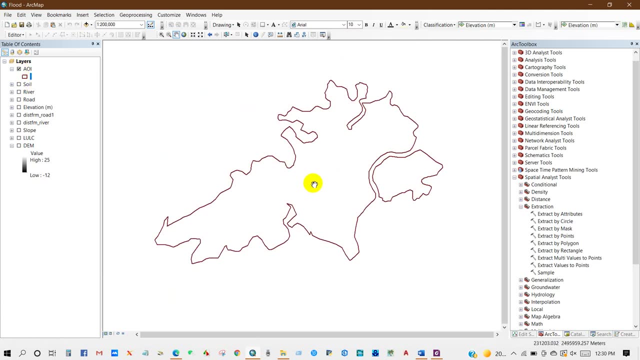 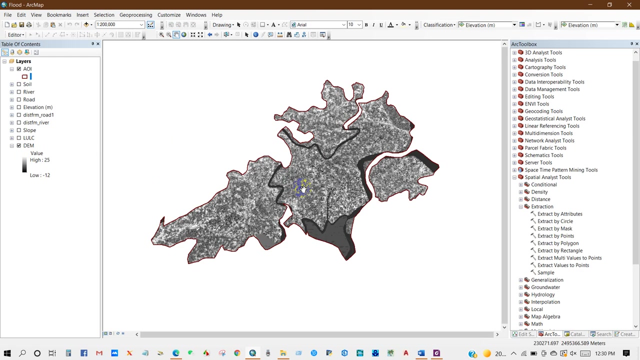 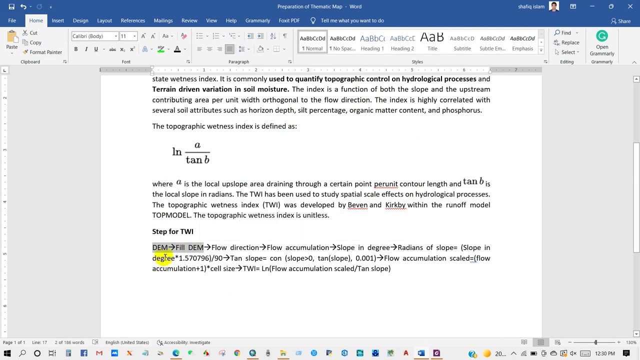 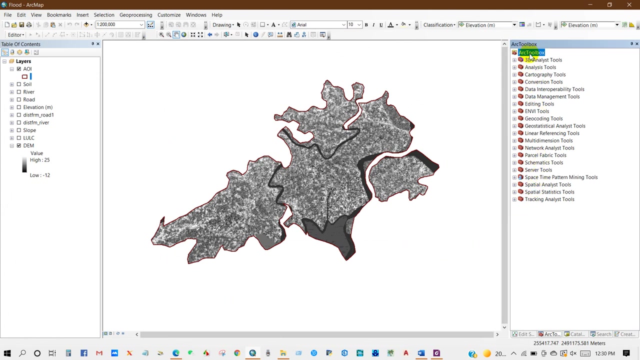 and here step for topographic witness index. first we need them. so go to arc map. here is our study area, area of interest, and here is our damn data, damn raster. so first we will perform, fill them. fill them for doing that. uh, go to arc toolbox and then spatial analyzed tools, and then hydrology. 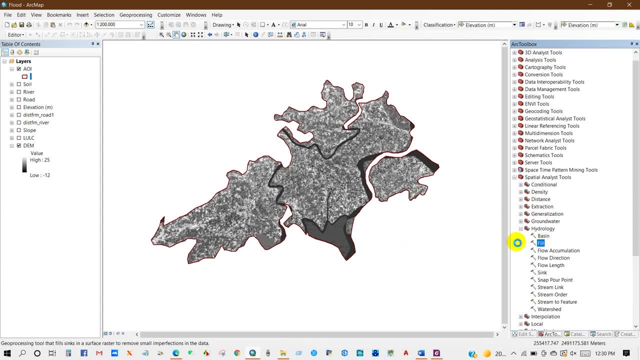 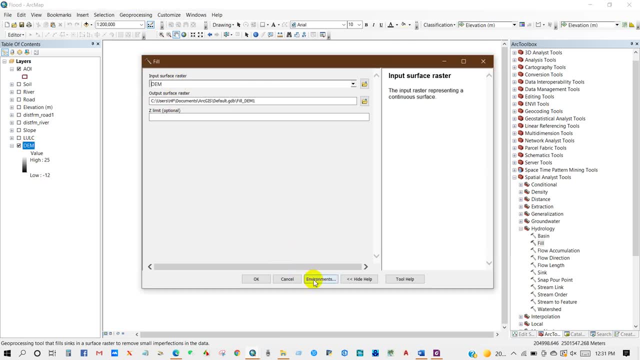 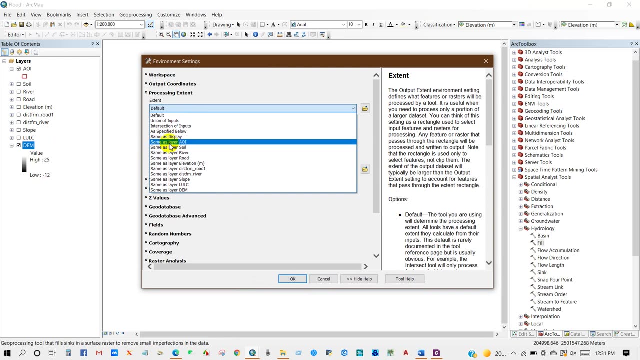 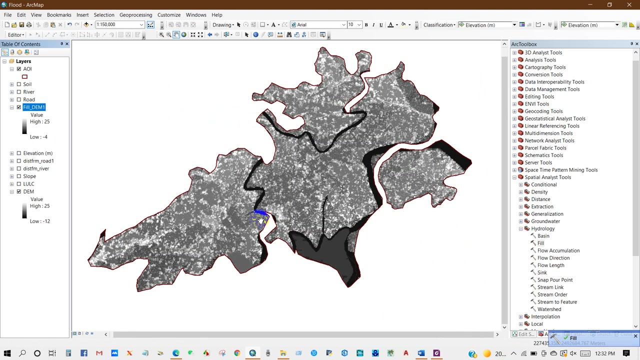 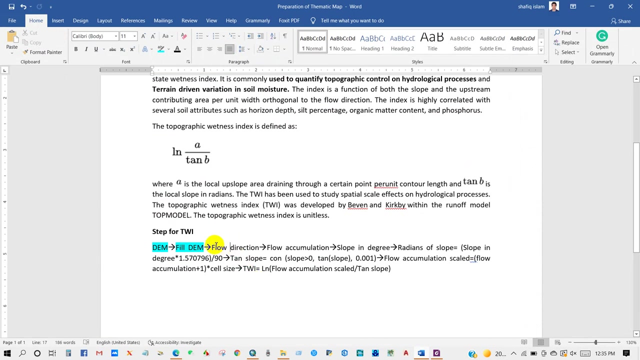 and then fill, double click on here and then add them as input surface raster and then environments processing extent. add uh, it will be as per area of interest, then okay. okay, field has been completed. now flow direction. now i will show you how to perform flow direction. click on follow. 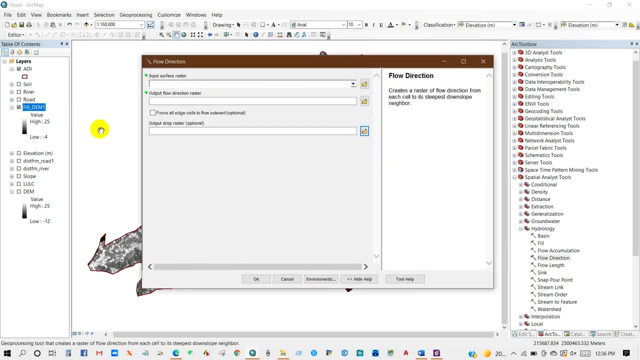 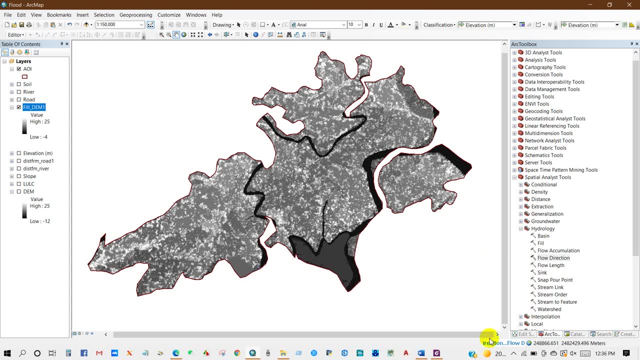 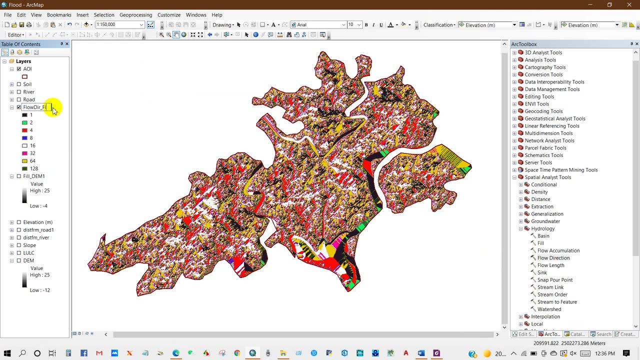 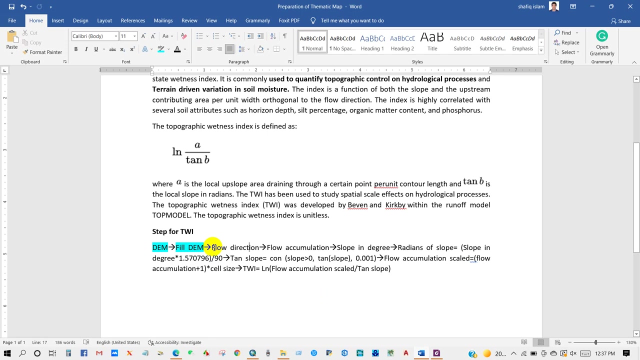 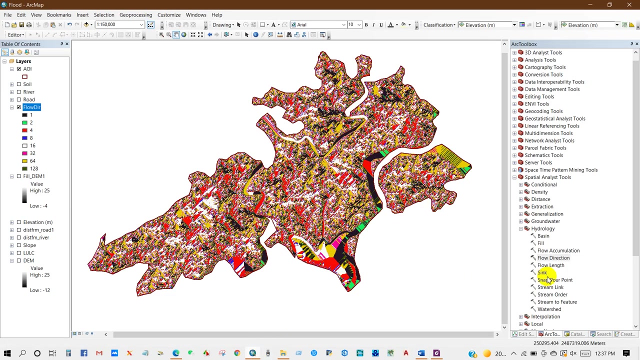 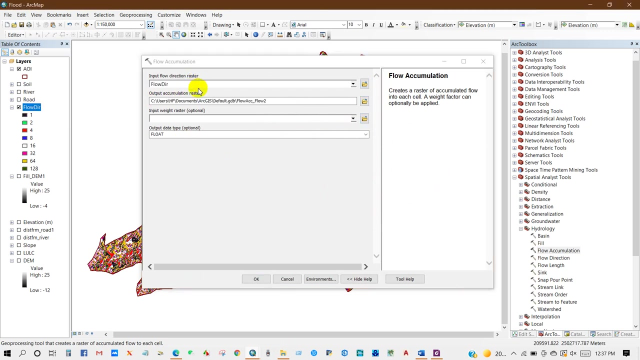 direction, another as well: input raster- input surface raster- will be filled in. then click ok, here is a flow direction. so flow direction has completed and now flow accumulation. click here flow accumulation. add flow direction in input flow direction raster, then output accumulation raster- i'm going to rename it flow accumulation- and then click ok. 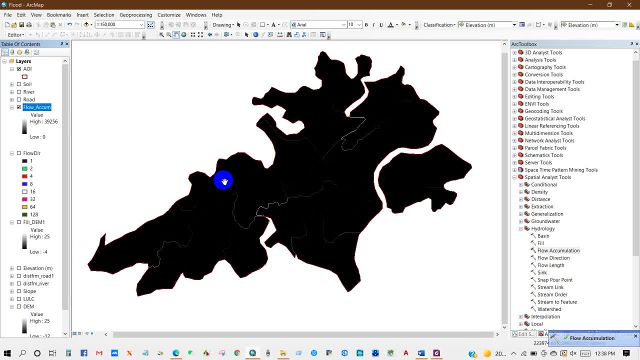 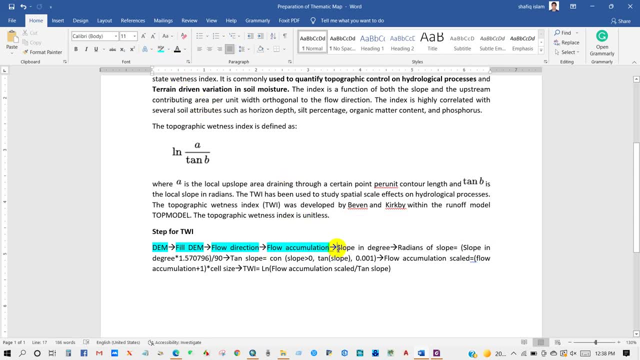 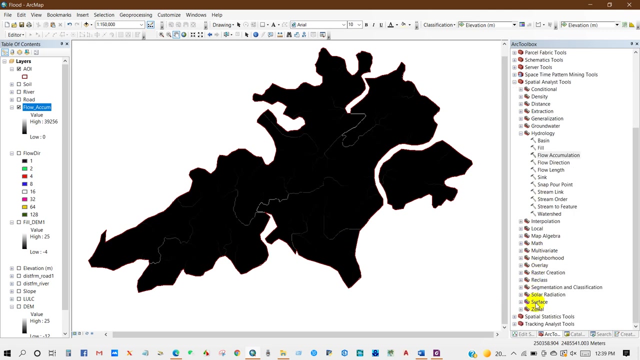 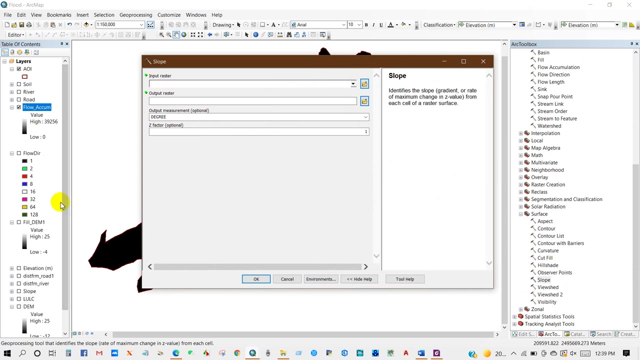 flow accumulation also has been done, so i'm going to rename it flow accumulation raster. and now, uh, slope in degree slope map for doing that. go to surface and here click on slope and input raster will be filled them as input raster, output raster and then output measurement will be degree. then click ok. 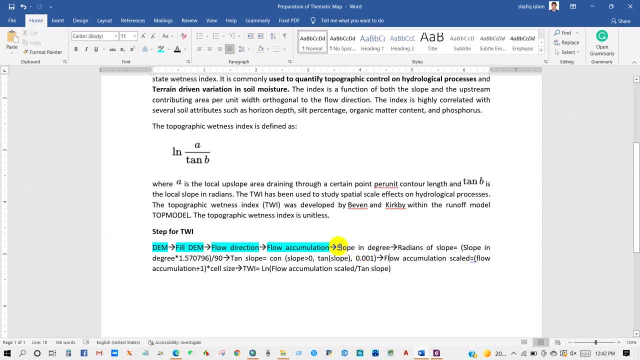 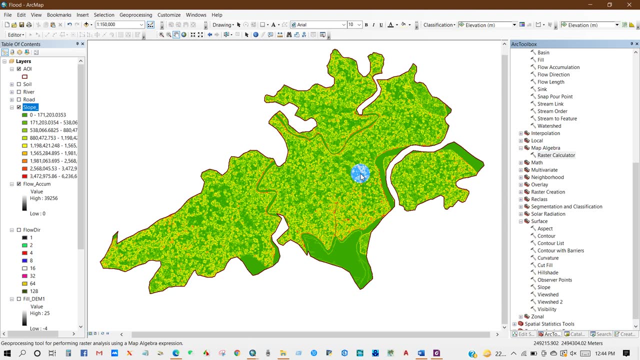 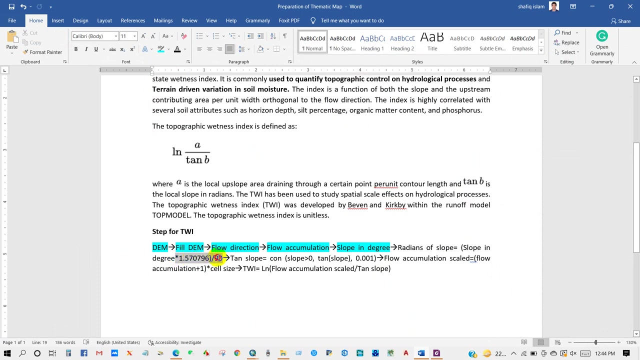 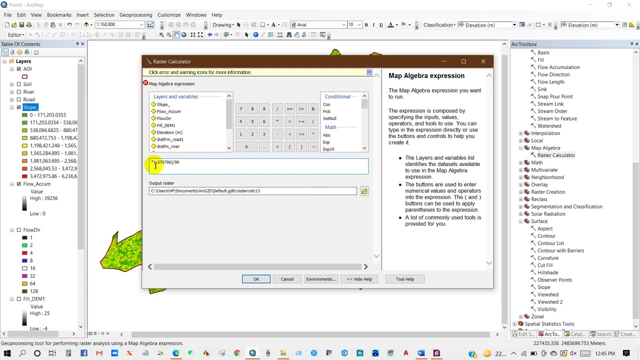 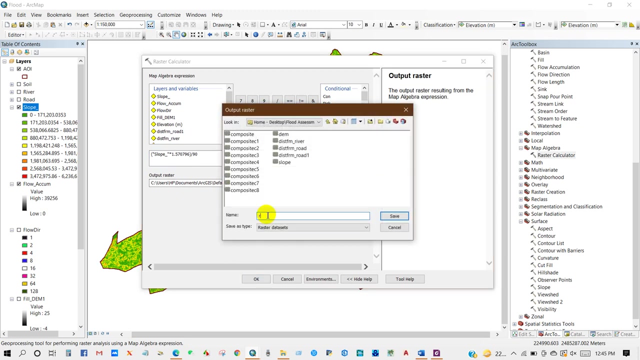 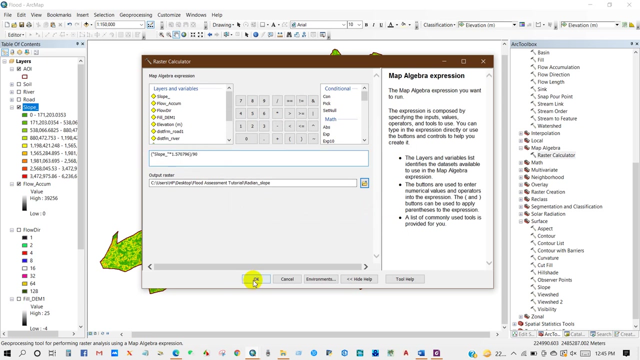 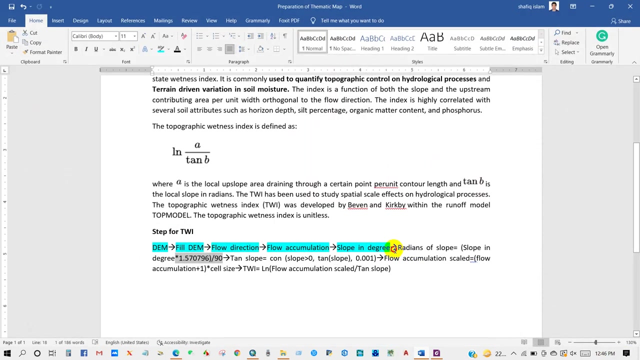 all our slope map has also done- and radius of slope. to do that go to map, algebra and then raster calculator. we have to add slope in degree, then this value and here add slope and i'm going to rename it as, uh, radial, radian of slope. it has done radians of slope and now 10 slope. 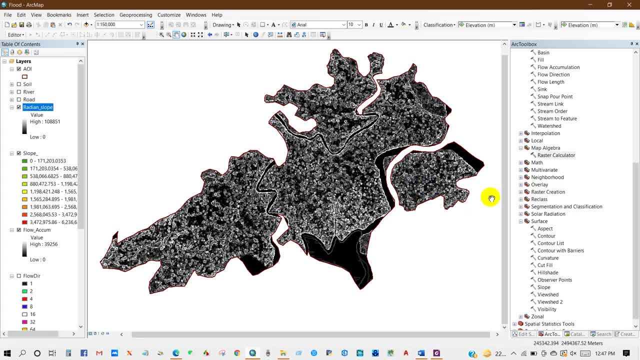 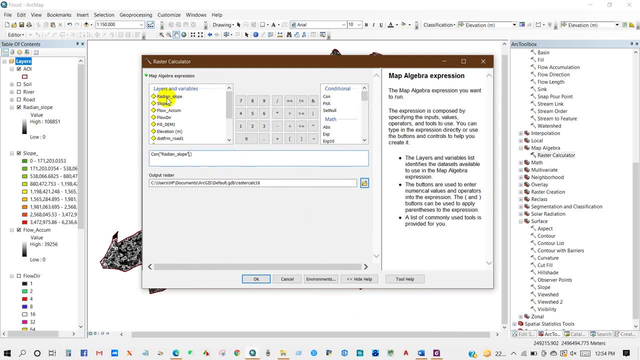 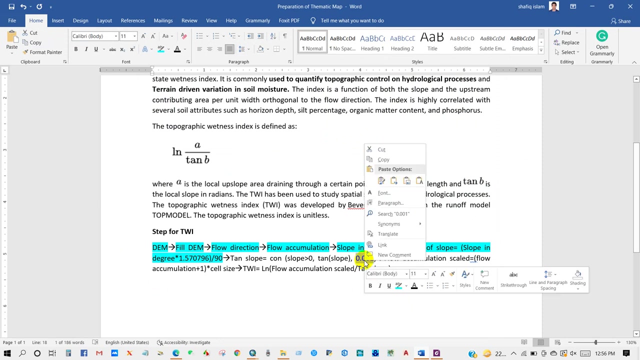 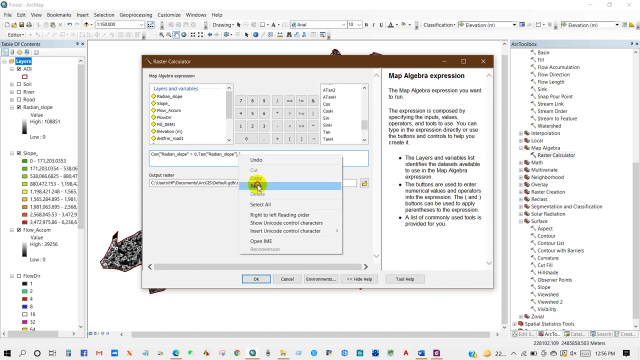 so you have to perform this 10 slope. for doing that, go to again raster calculator and then condition radian slope, then greater than 0, then 10, then radian slope, and here put the value point 0, 0, 1, 0.001. 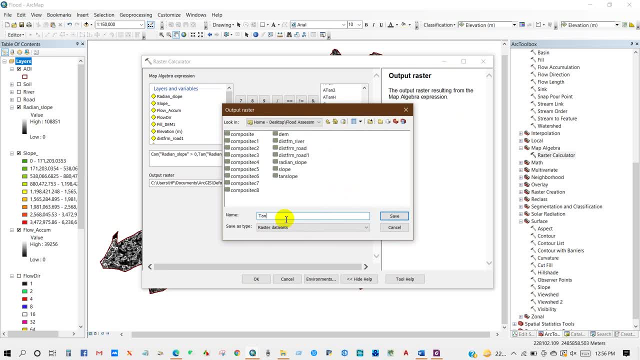 r2 raster. you can save output raster in a r2 raster. you can save output raster in a folder where you want to save, folder where you want to save, and i'm going to rename it as 10 and i'm going to rename it as 10. 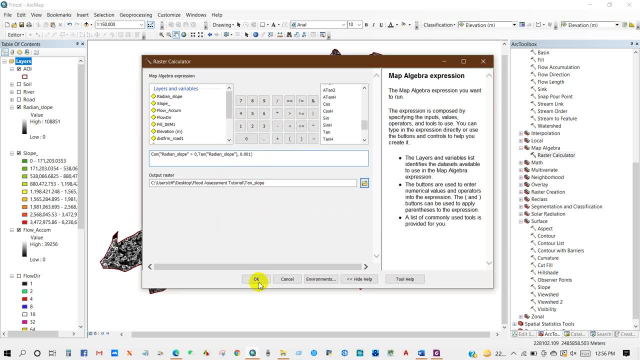 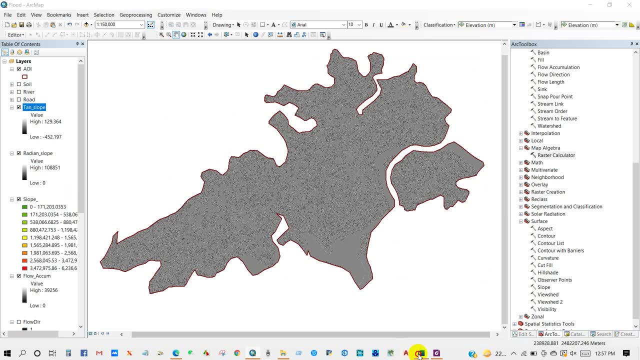 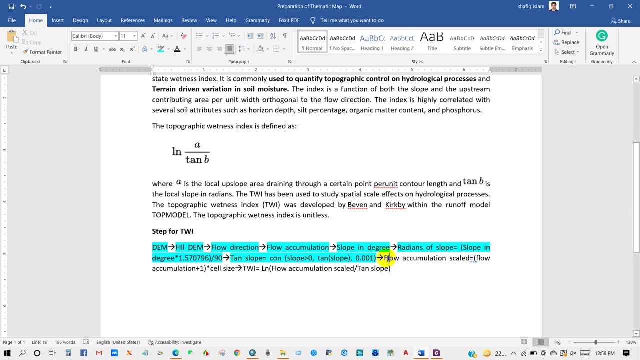 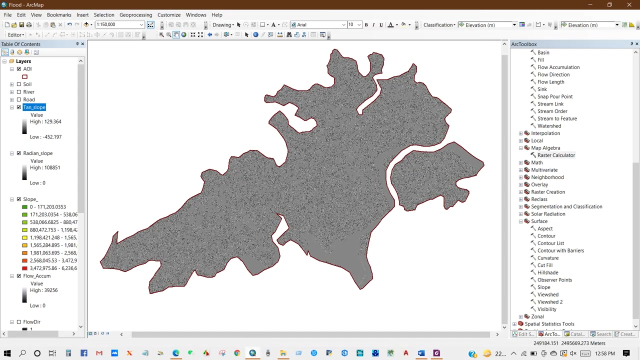 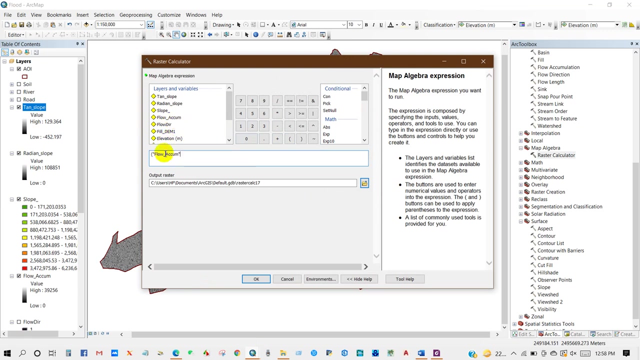 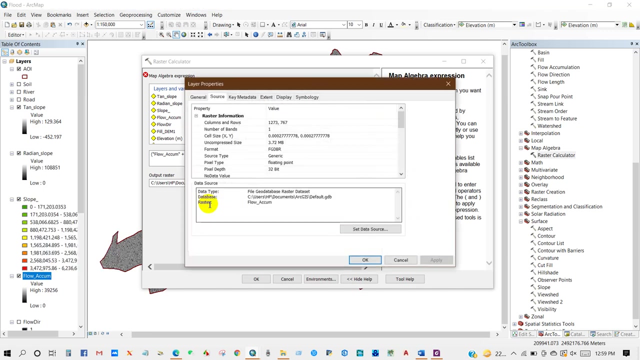 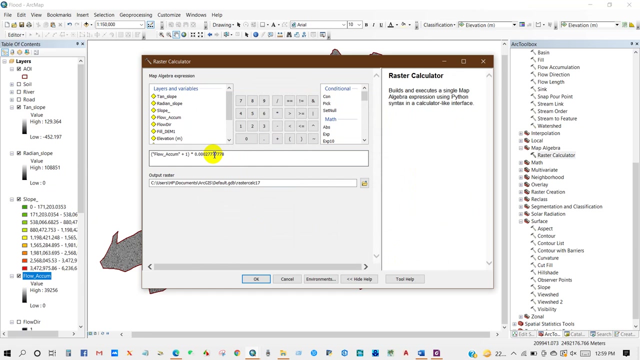 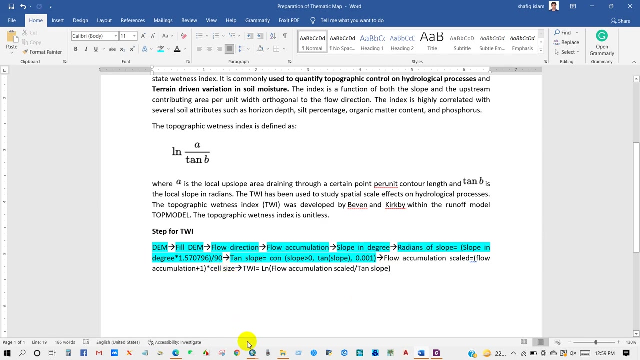 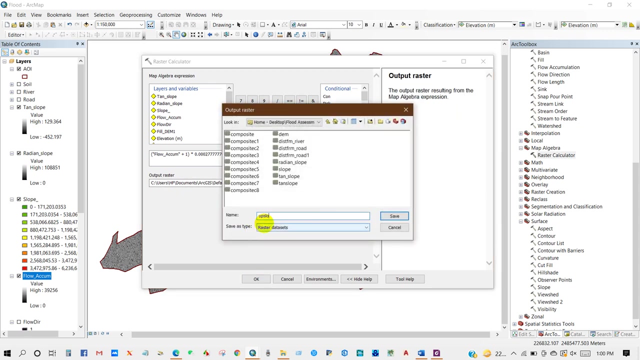 slope, slope and click ok, so tan slope has been done. and then flow accumulation is scaled again. go to raster calculator, first bracket and then flow accumulation plus one first bracket close into go to flow accumulation, then copy the cell size and paste here cell size output raster. i'm going to uh rename the output raster as upslope, then save, then okay. 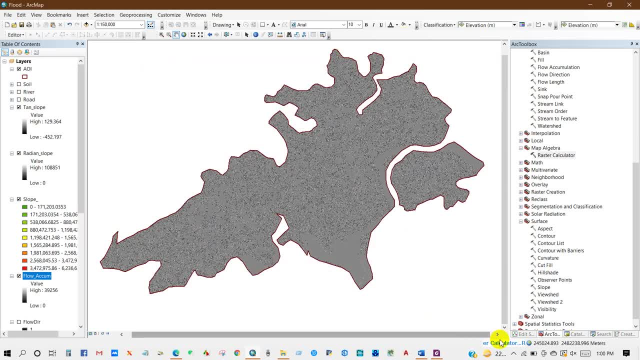 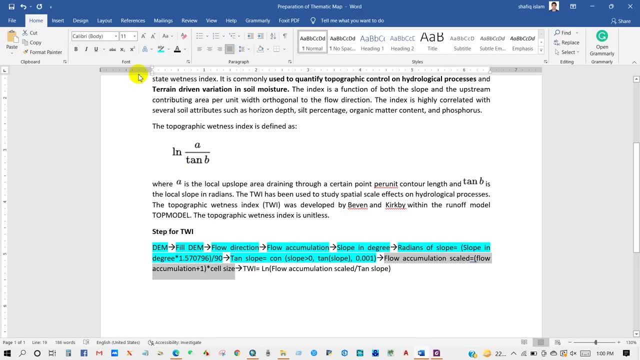 upslope has been done, i mean flow accumulation is scaled. and then, finally, topographic wetness index. so for doing that, i'm going to rename it to topographic wetness index. so for doing that, i'm going to rename it to topographic wetness index. 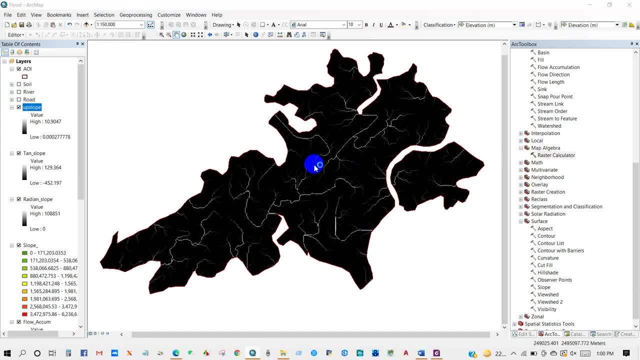 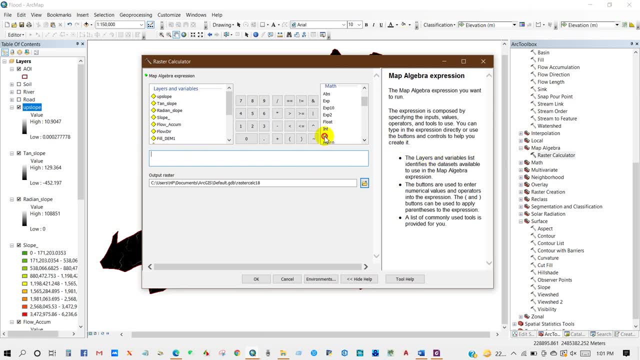 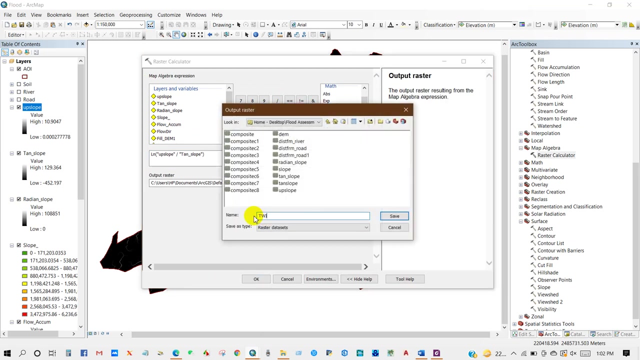 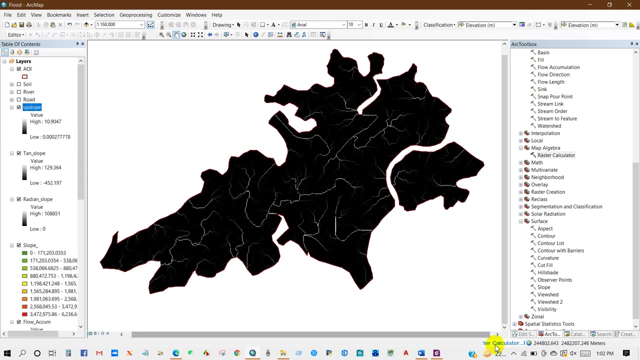 you have to perform this equation. go to raster calculator, then lon up slope slash, i mean divided by tan slope output raster. save output raster. i'm going to name as twi topographic wetness index and then click ok. so our topography goodness index has been done. 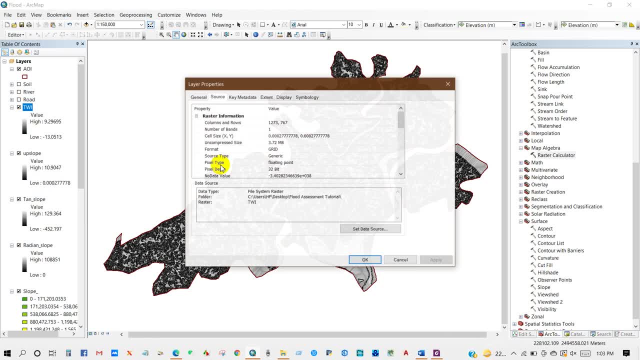 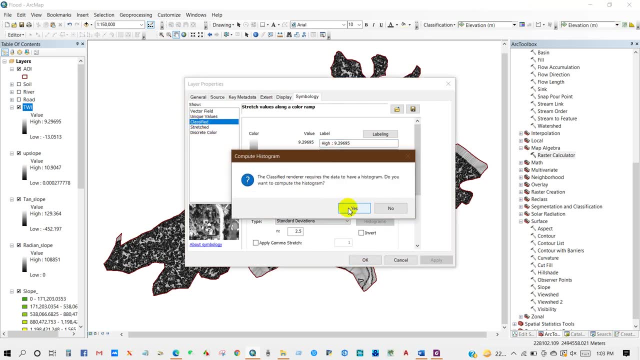 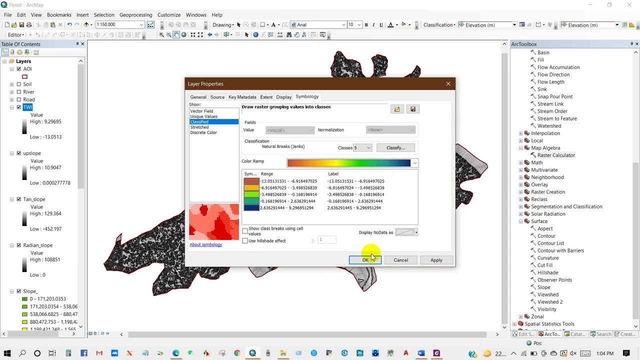 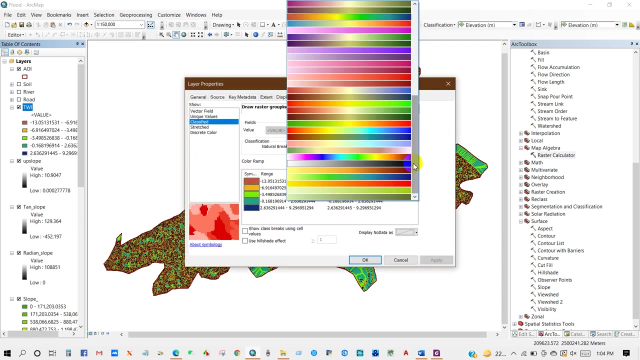 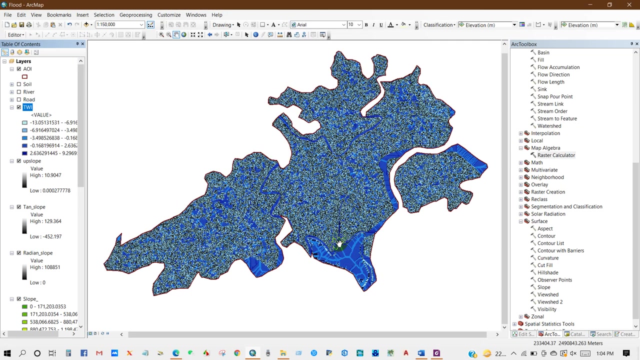 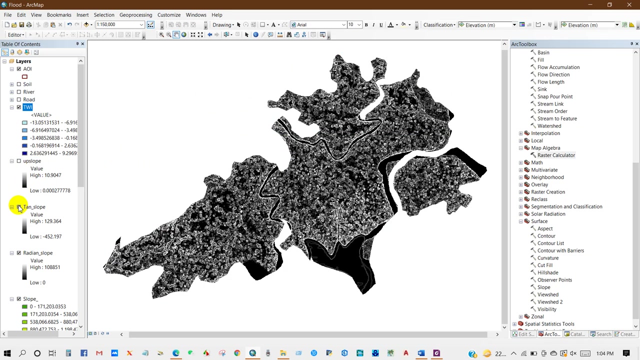 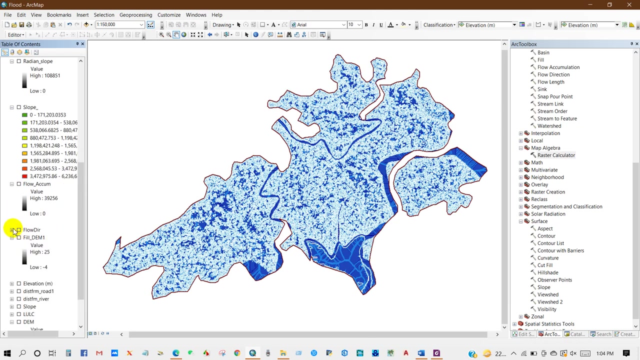 now you can classify it, go to properties and then symbology classified, you can change the color, Sitcom, you can change the color according to your preference. You can change the color according to your preference. Now i don't need this data flow direction, flow accumulation or absolute, so i'm letting this flow direction flow large up slope. so there are many. 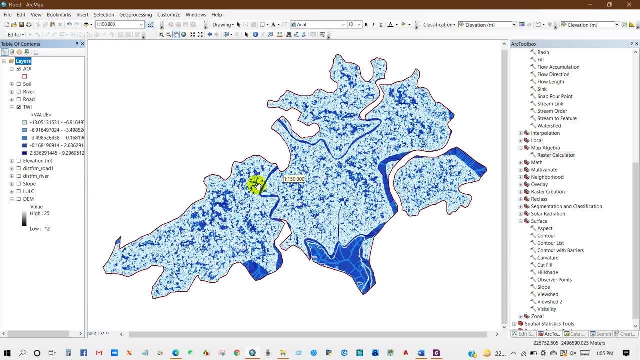 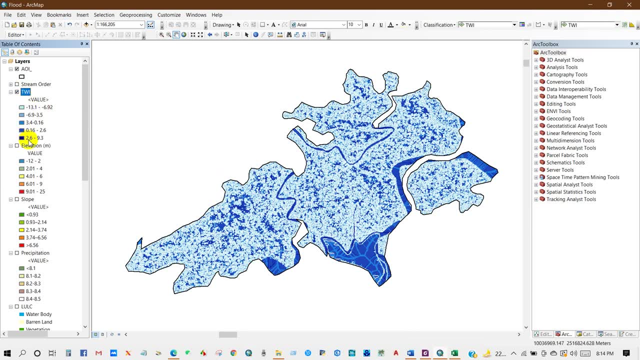 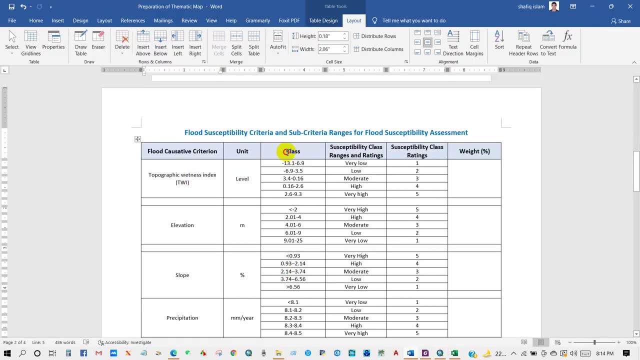 So I don't need this data flow direction. flow accumulation help slope, so I'm letting this, this raster, so our topographic witness index has done so. we have got all the thematic maps here. now we can see here topographic index, then class, and according to class value. i have arranged here susceptibility, class ranges and ratings. 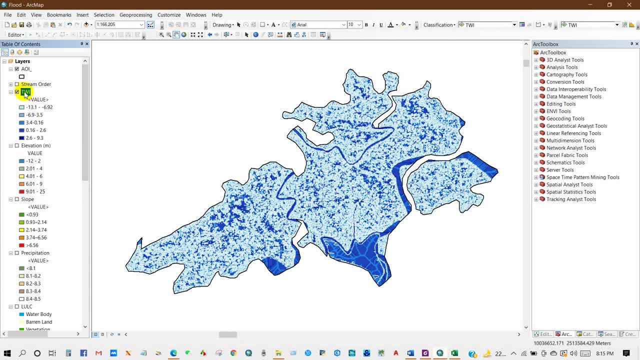 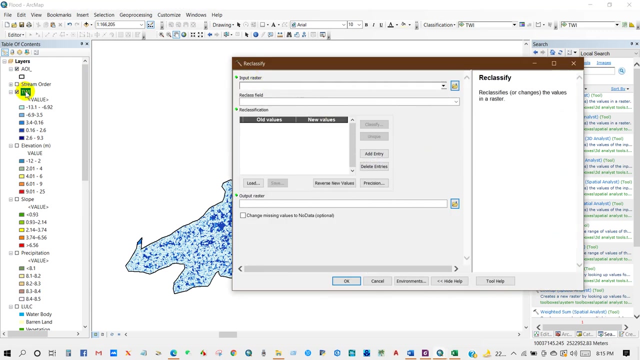 i will describe one by one. in order to combine the data set, they must be in a common scale. we have to reclassify all the thematic maps and need to be organized: one to five scale for each factor. classify input raster, add topographic witness index and then old value and new value. 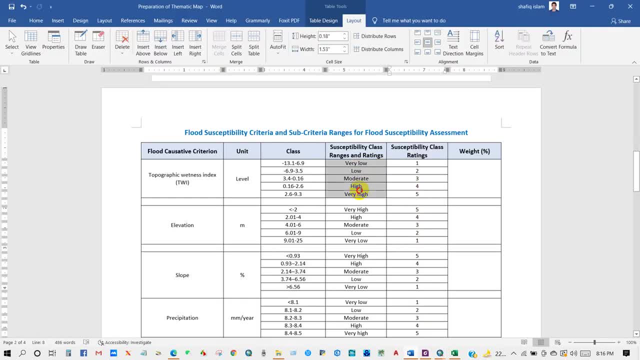 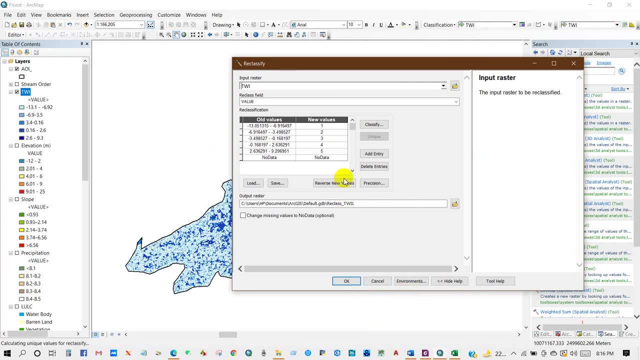 so topographic index. the lower value means very low probability for flat. very low, true, very high. so it will be one, two, three, four, five and then output raster. i'm going to rename it topographic witness index and then output raster. i'm going to rename it topographic witness index and then output raster. 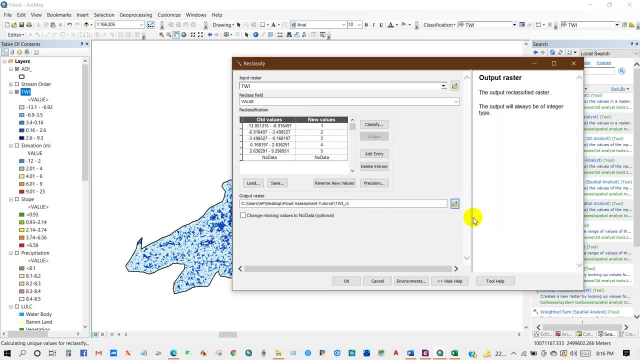 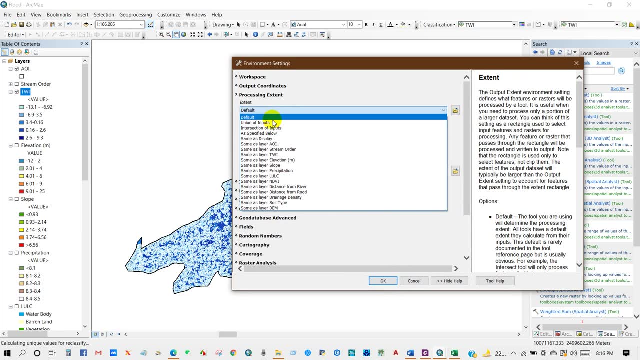 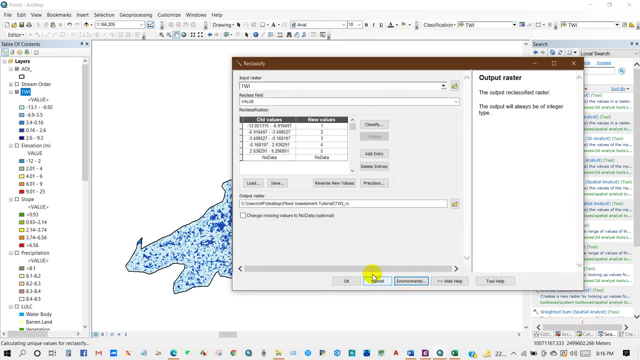 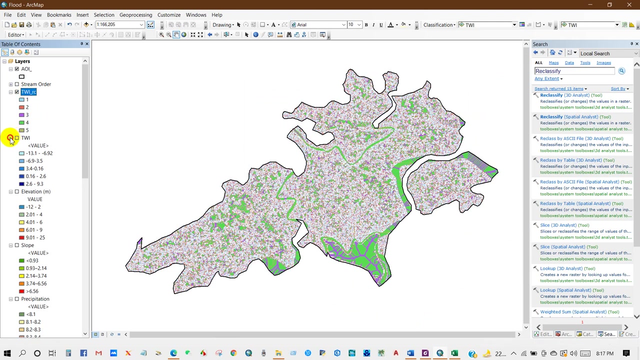 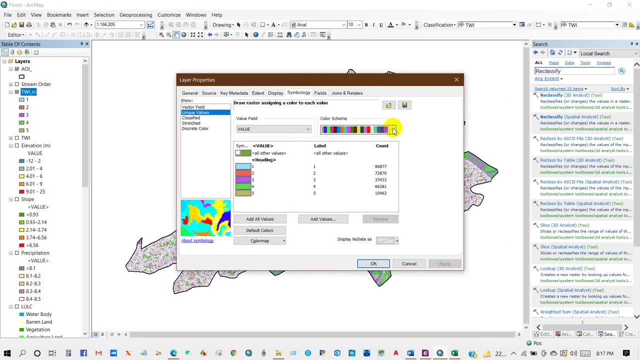 Boris, you are reclassified. you will get an rc. then click save. environment processing extent will be the area of interest. raster analysis- uh. it will be masked. mass data also will be area of interest. then click ok. okay, so topographic witness in this uh data has been reclassified one to five. you can change the color. 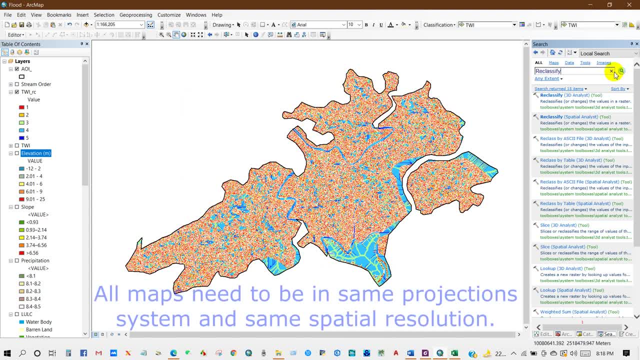 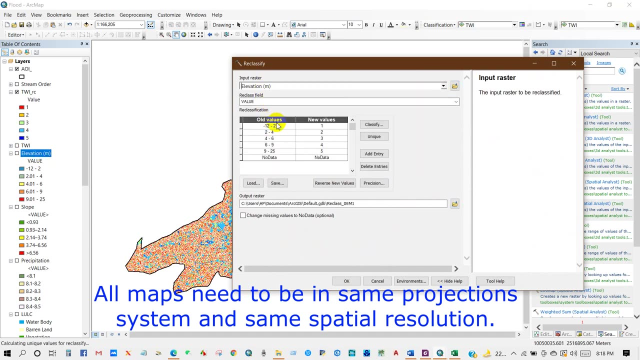 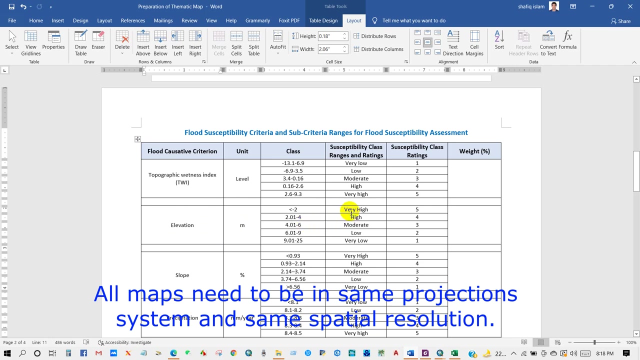 then elevation, again reclassify, click here, reclassify and add elevation as input raster and then, uh, all value and new value. so for elevation, lower value means very high probability. for flat i mean, uh, lower lower value to higher value, that means very high to very low product probability. so five, four, three, two, one, it will be the class range. 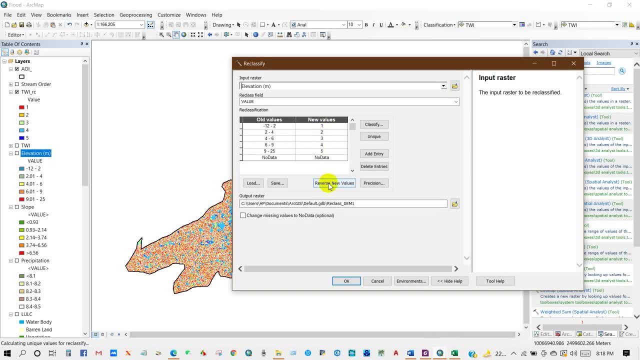 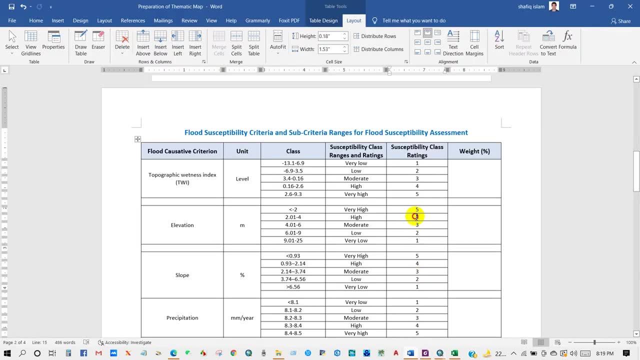 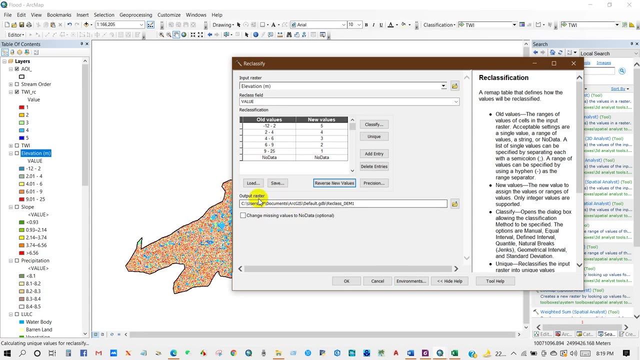 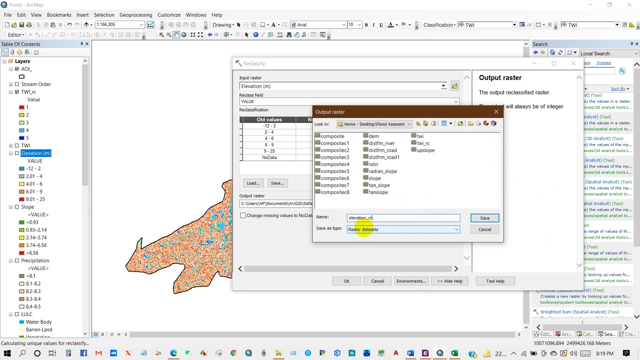 so it will be five four, three, two, one. reversed new value: five four, three, two, one. very low value means um for elevation is higher flood susceptibility. then output raster, save our raster. i'm going to give it a name: elevation, reclassified rc. then save and then click ok. 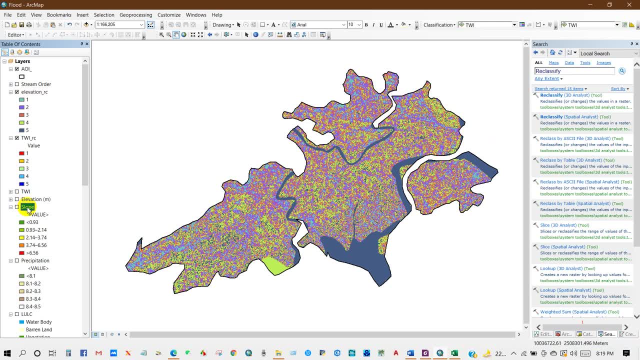 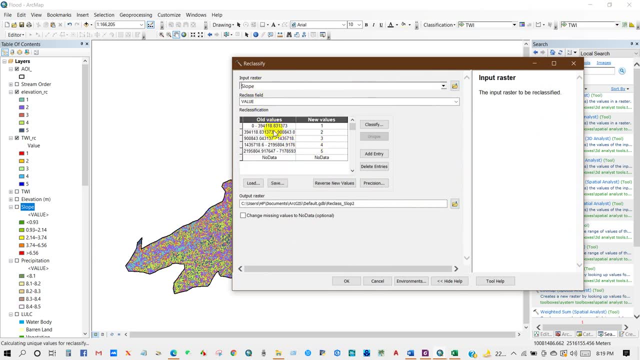 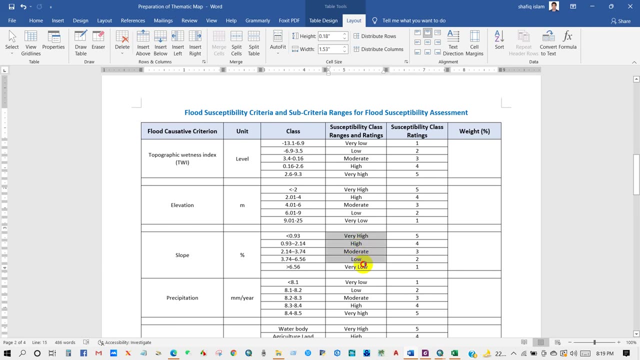 elevation raster has been reclassified, and then slope and again reclassify input raster, slope and then uh. the new value will be for uh. for slope, lower value to higher value means very high to very low flat probability. so it will be uh. five, four, three, two, one lower slope means uh. 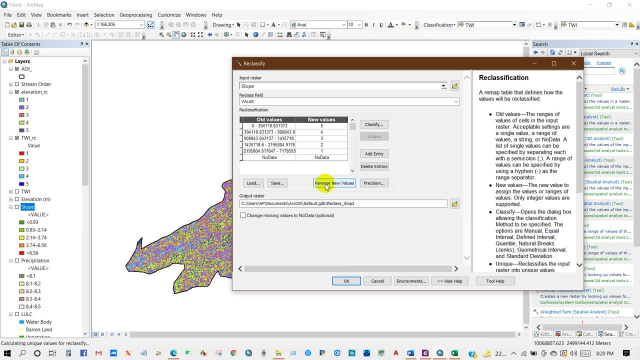 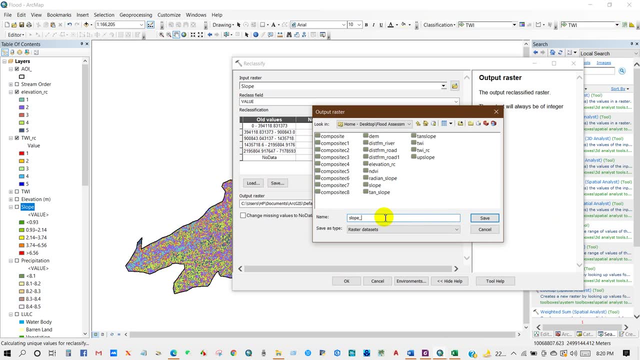 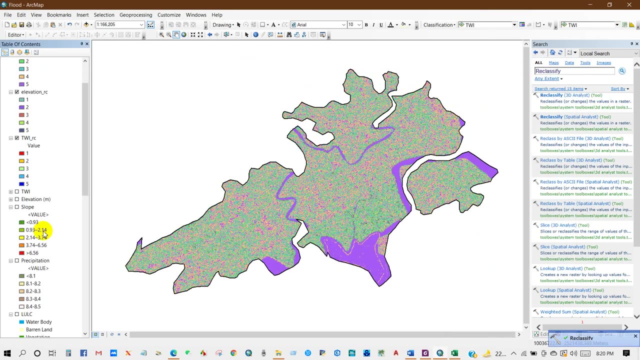 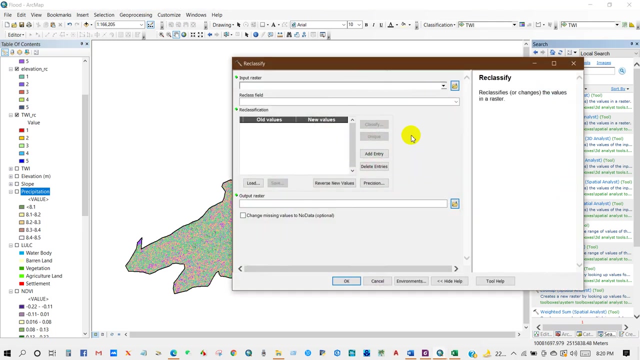 very high flood probability. it will be reverse: five, four, three, two, one. save the output raster. slope, rc reclassified, so slope has been done, reclassified and then precipitation, reclassify again. input raster will be uh, precipitation, and then for value, new value, so for precipitation. so lower precipitation means very low for probability. 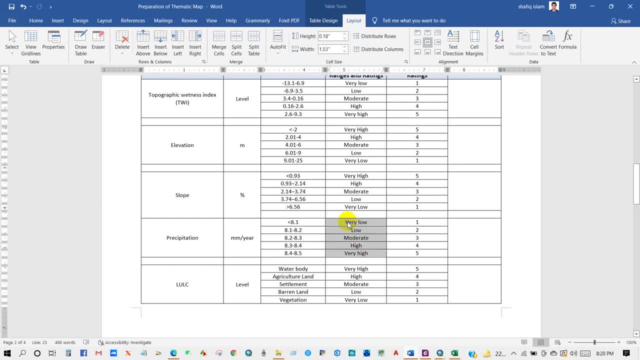 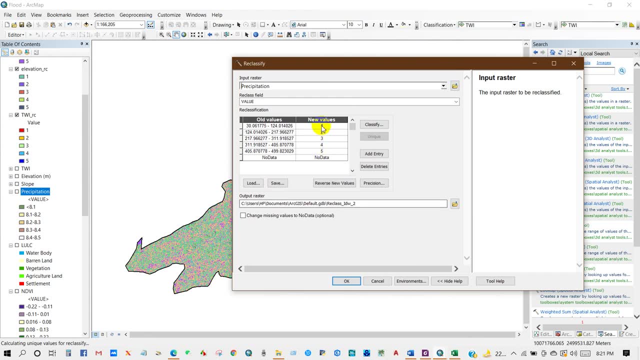 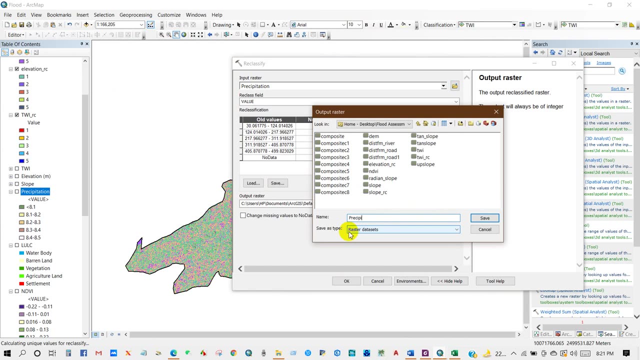 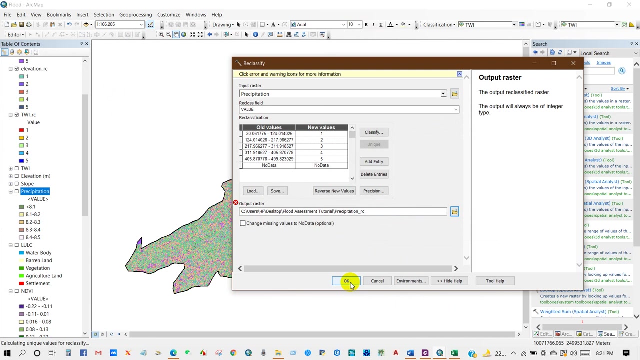 so lower to higher precipitation means very low to very high probability for flat risk. so it will be okay on two, three, four, five low to high, and then uh, rename the reclassified raster for precipitation, precipitation rc, then save, and then uh, there's a problem. output raster the length of the grid mean maybe it is too long. 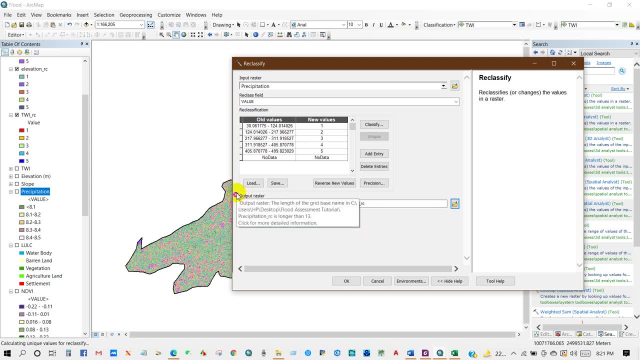 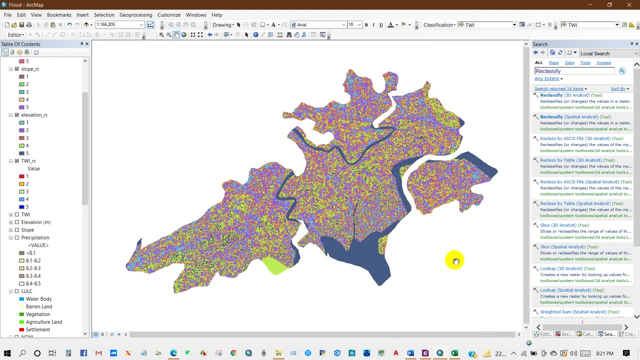 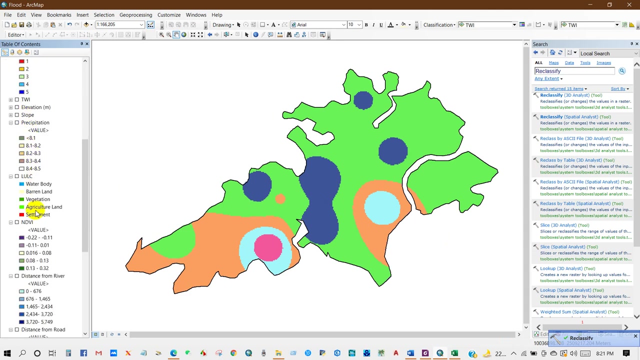 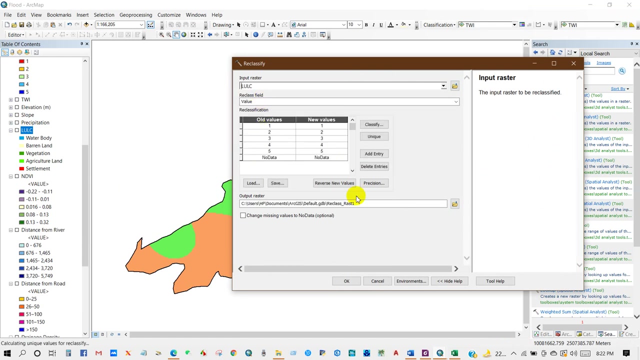 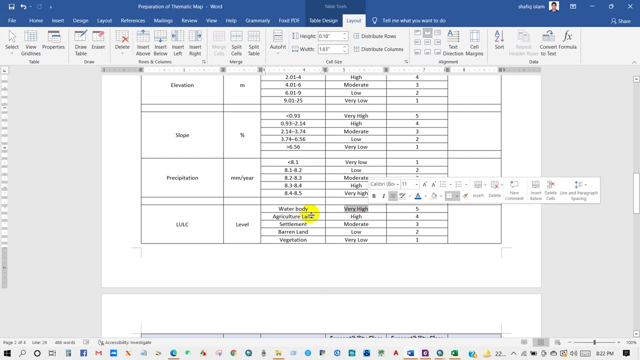 the name. so i'm going to decrease this and then i think it will be okay. yeah, okay then, okay. so precipitation- reclassification has done and i have show Free seven plus photos- is a higher probability for flood water. moderate water body- uh, water谢 water body- a very high probability for flood. so it will be five. 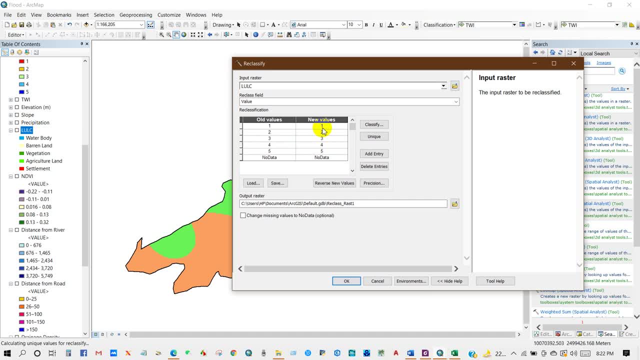 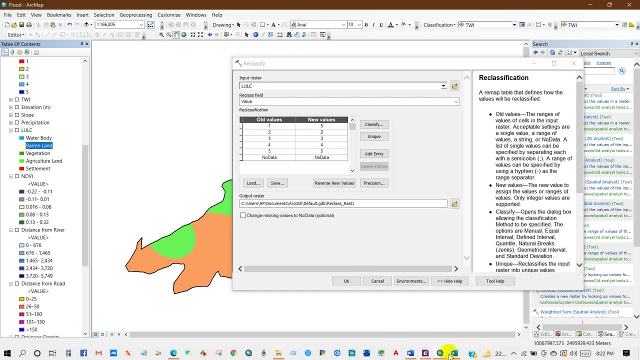 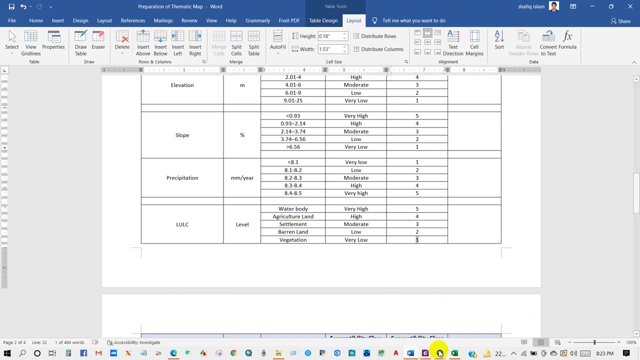 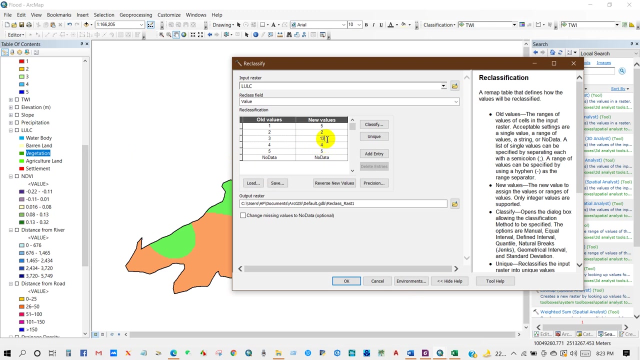 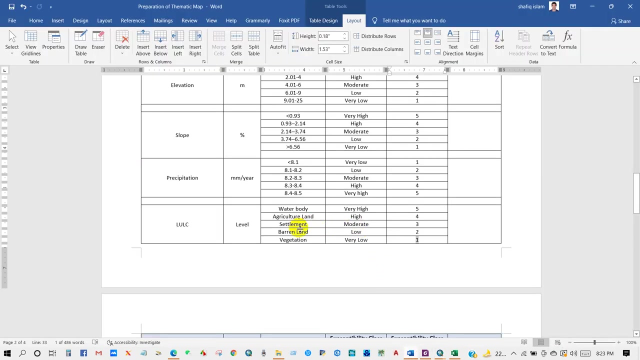 so one, uh, it will be five. then two: barren land. barren land will be low, comparatively low for flood risk, comparatively low in terms of this classification. then vegetation will be very low, so it will be one, and then for agricultural land it will be high, so the rank will be four. 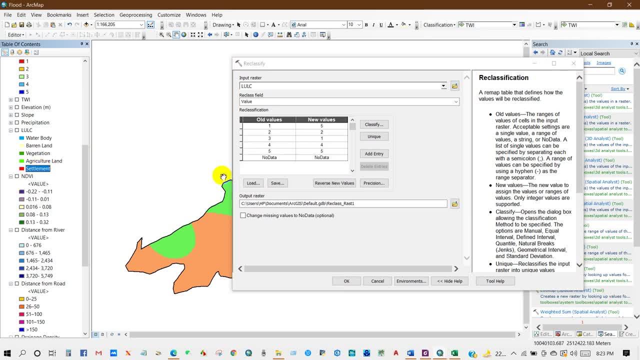 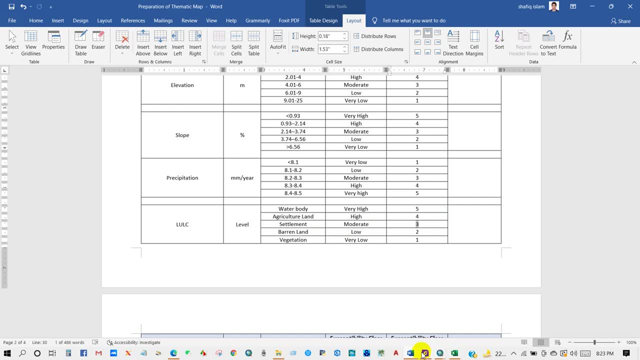 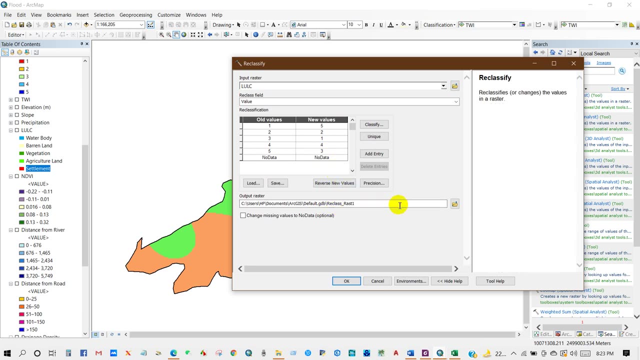 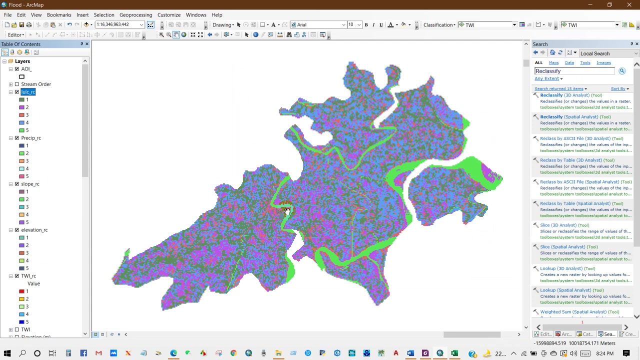 it is already four, then five. settlement: settlement: moderate for flood risk: here uh five, it will be uh three. then output raster: save. output raster lulc rc, then save and then okay, um, lulc has been classified, reclassified. and then ndvi, normalized difference vegetation index. so add ndvi as input raster. 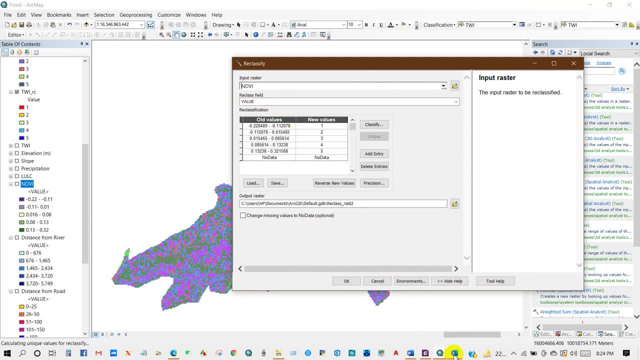 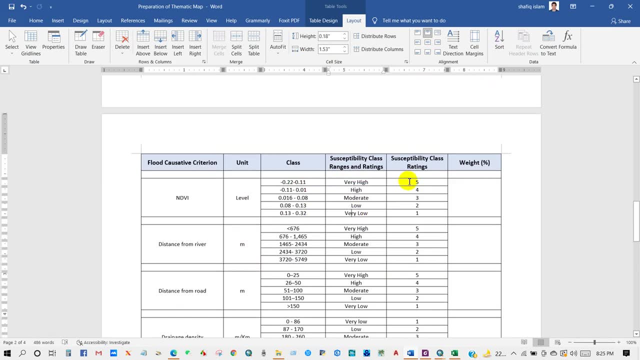 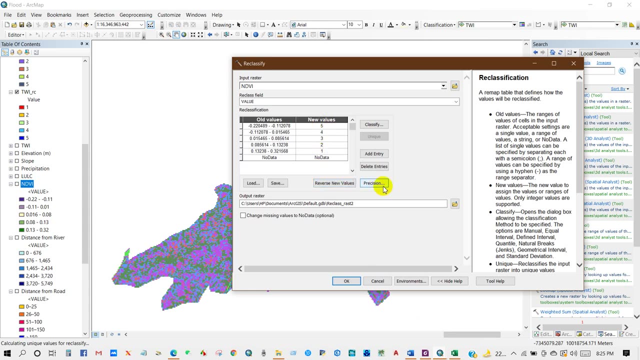 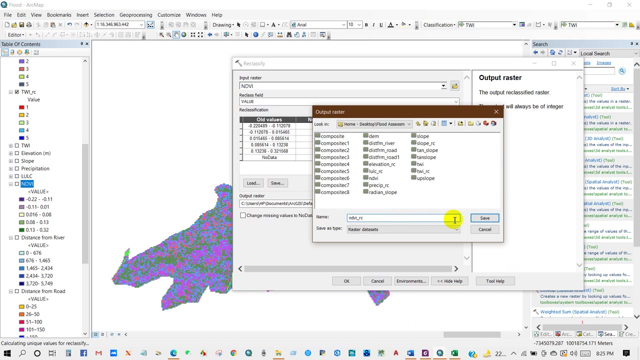 and then new values. so for ndvi, lower ndvi to high ndva means very high to very low flood probability, so it will be 5 to 1, the reverse. new value 54321 and then output raster. rename ndvi reclassified, then save okay. 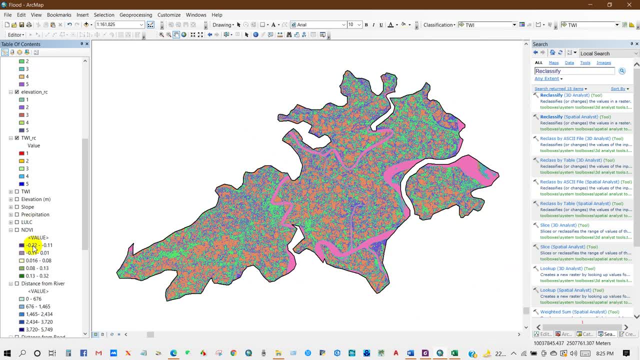 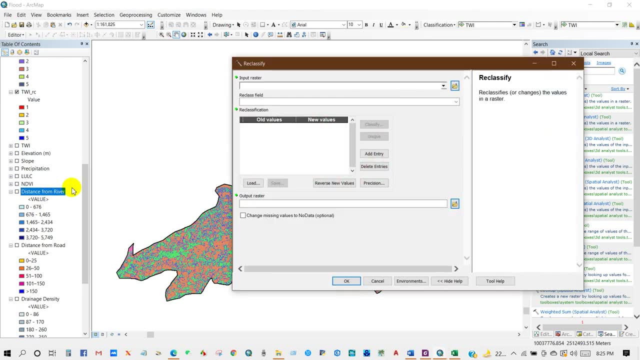 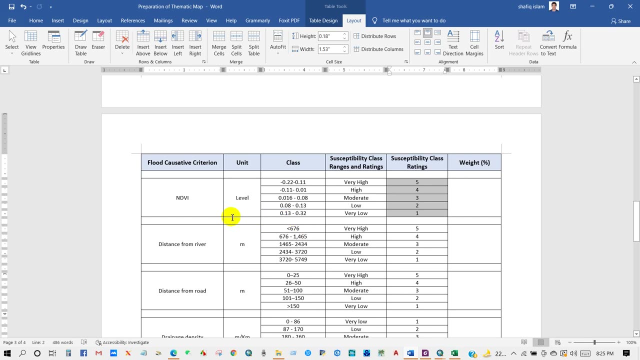 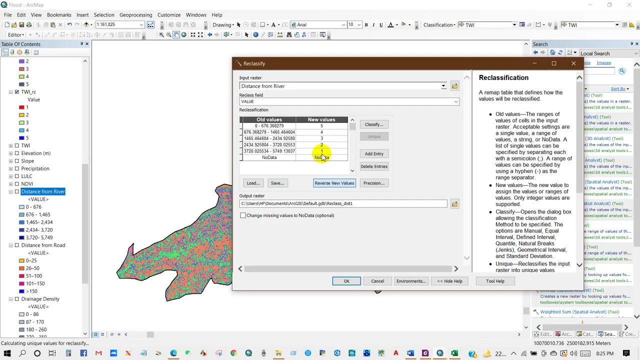 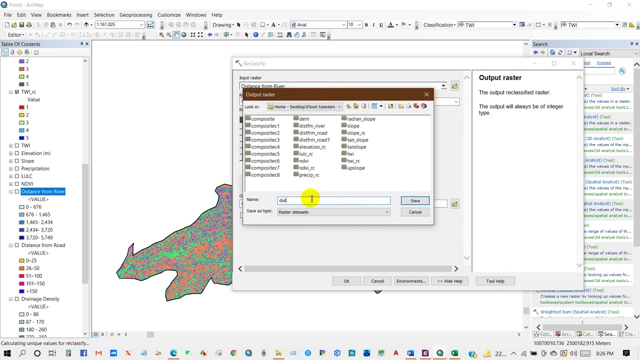 so our ndvi has been reclassified. and then distance from river: reclassify input raster- distance from river. and then value for distance from river: uh, very low to very high distance. it will be very high to, uh, very low probability. i mean closer river distance means high. 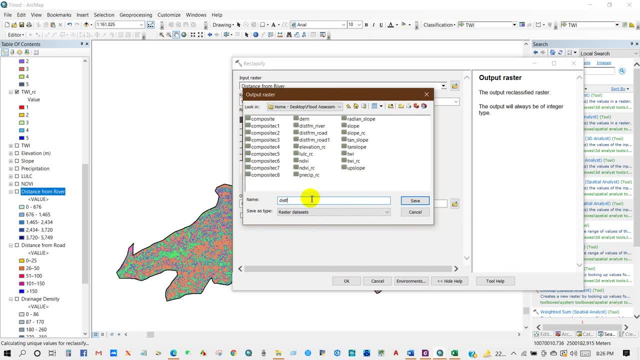 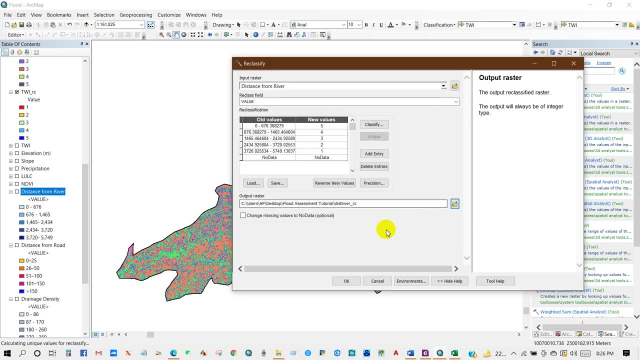 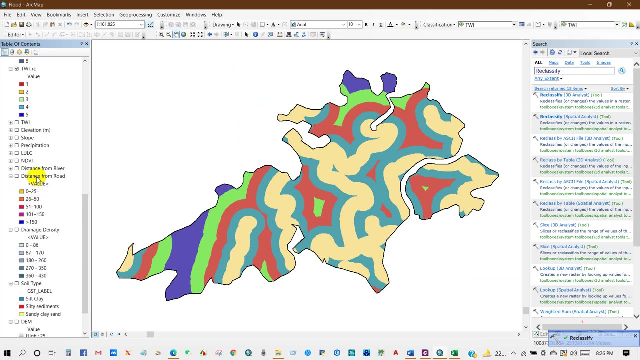 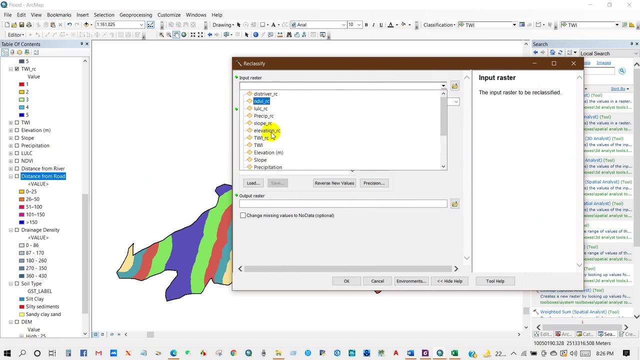 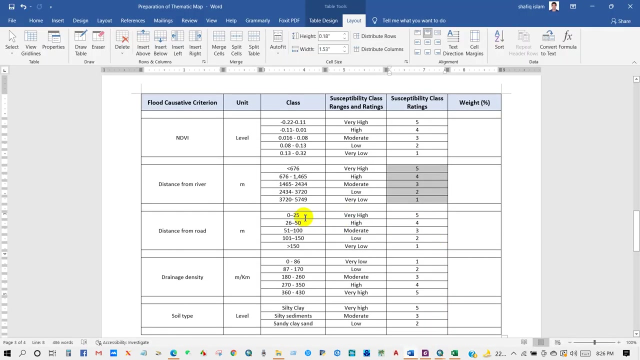 probability for flood. and okay, so distance from river, reclassification has done, and then distance from road, again reclassify, and then, for distance from road, lower value to higher value. i mean lower distance to higher distance, very high to very low. so five four, three, two, one. it will be reversed: five four, three, two, one. then. 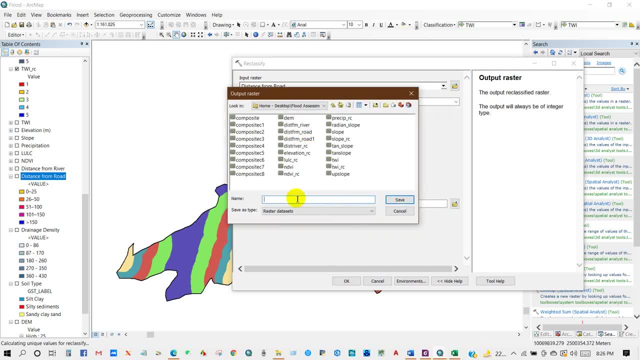 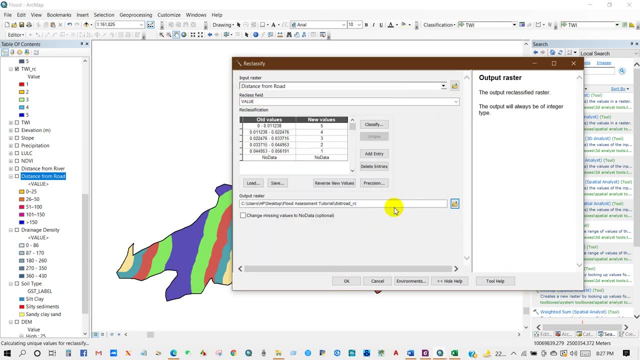 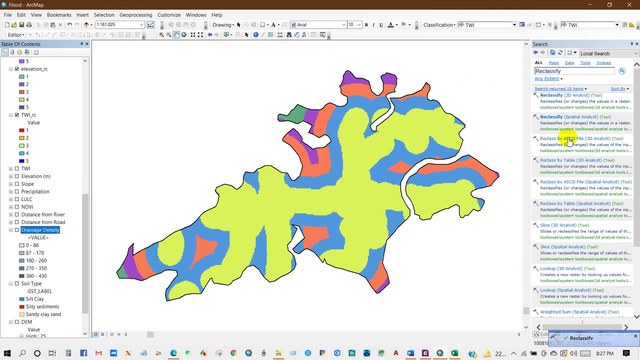 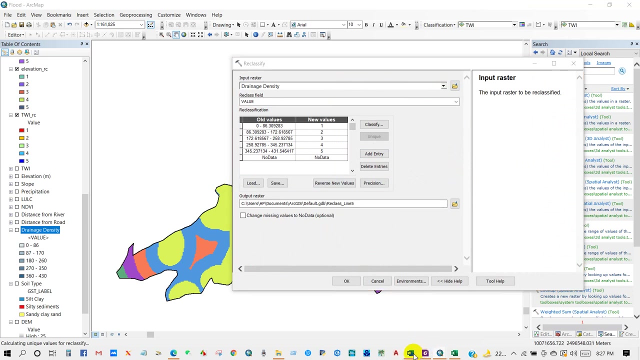 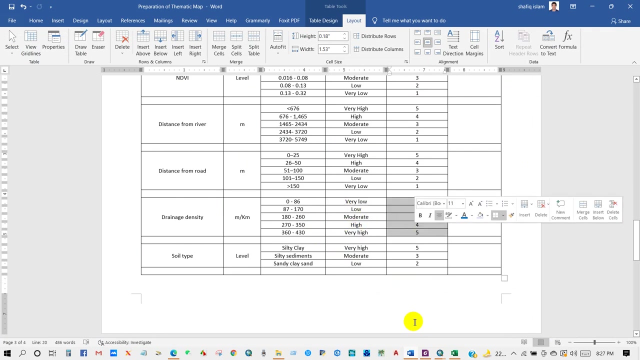 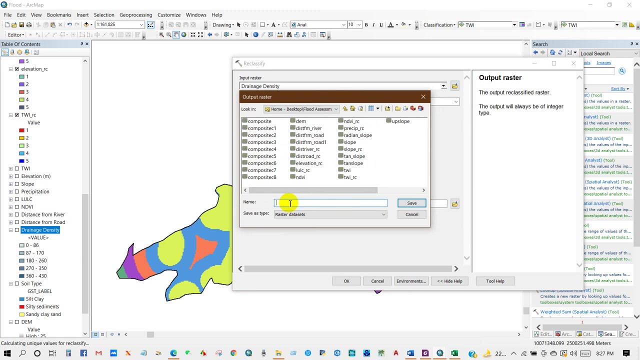 output raster: save output raster and rename save and then okay, so distance from road has been done. then drainage density, again reclassification input raster as drainage density, then value for drainage density: lower drainage density means a very low flood probability. higher drainage density mean high flood probability. then rename drainage density and then reclassification rc. 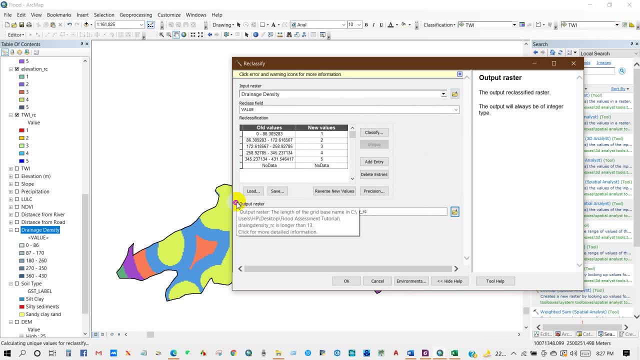 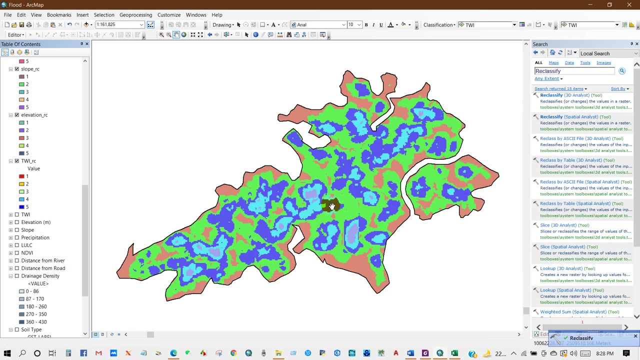 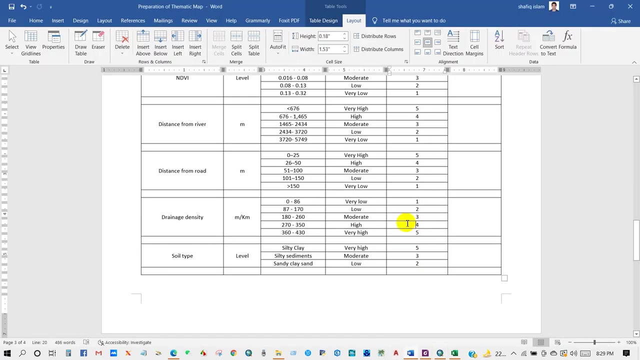 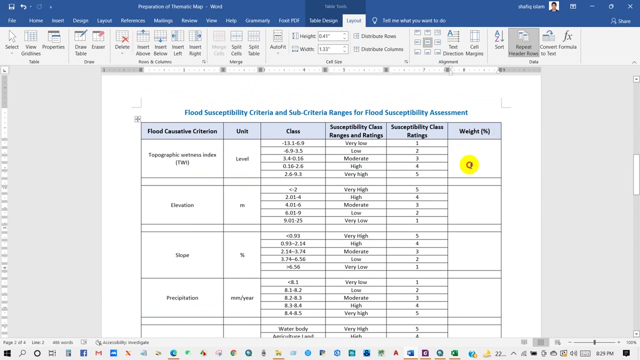 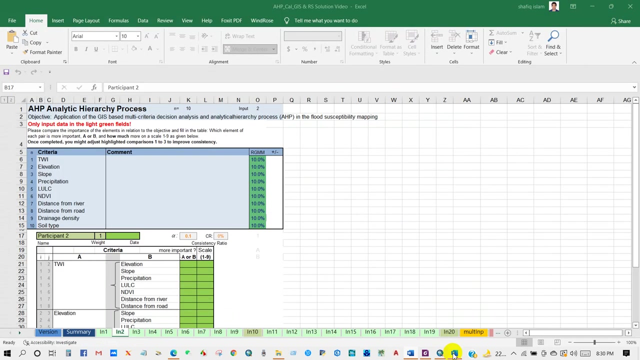 save. maybe the name is too long now i think it will be okay. yes, then okay. so already, density classification has done so. our all thematic map reclassification has done in a scale on to five. now i will show you how to calculate thematic map weight using uh, asp excel sheet for js input. so here is our asp excel sheet. 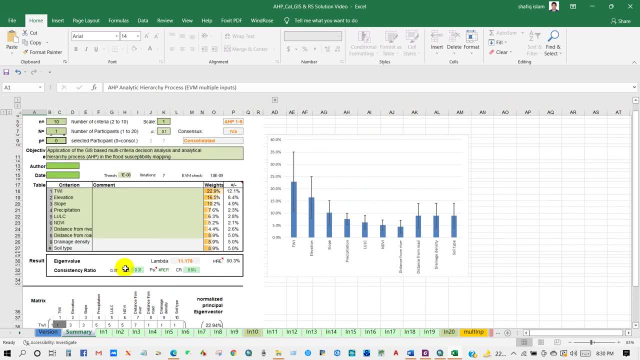 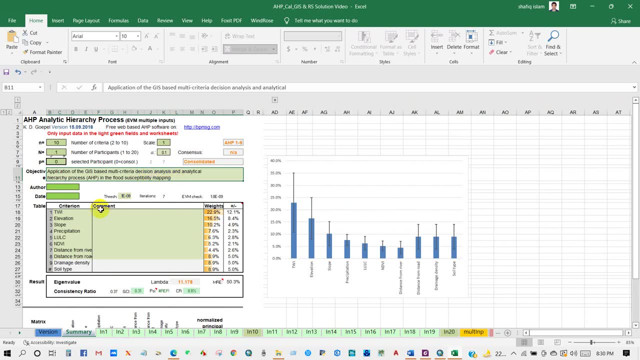 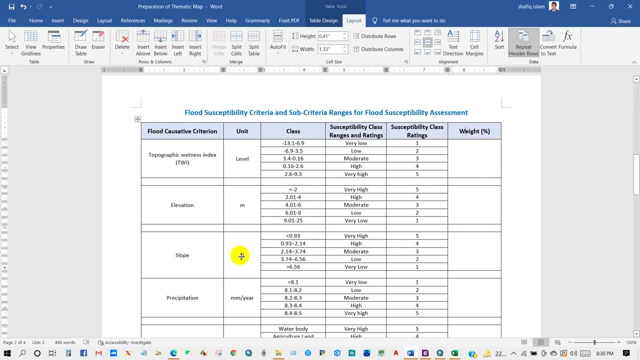 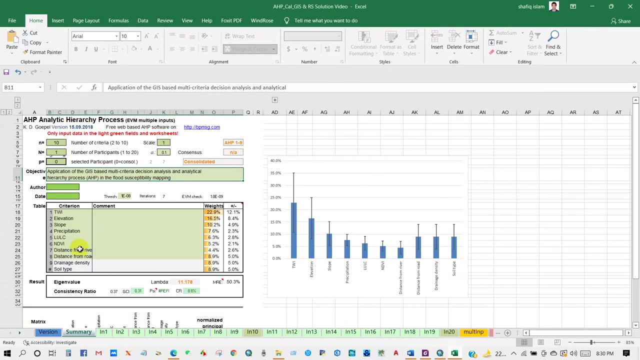 here, uh, you can write of your study title in objectives section and here in the flat criteria write the wall criteria. here i mean all the factor elevation, slope, level c and all the factors you have to write here. and then here you can see the criteria i have written here. 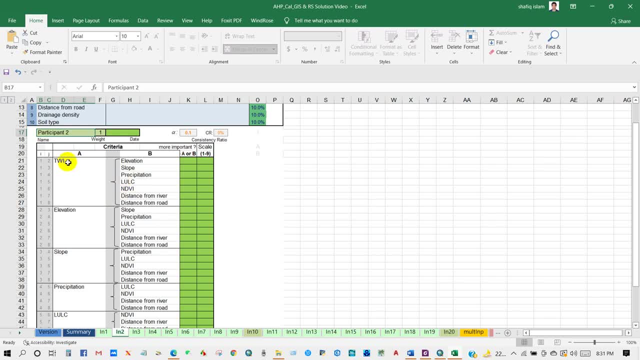 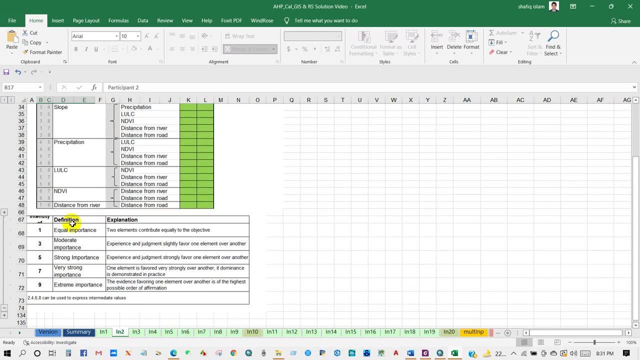 and then this criteria box. you can see here criteria a and b. i mean uh more important, what is important, a or b, and then a scale one to nine. scale one equal importance, three, five, seven, nine, the category of scale, and here you can see what is uh important. categorical box is one, two, nine. scale one, two, nine. 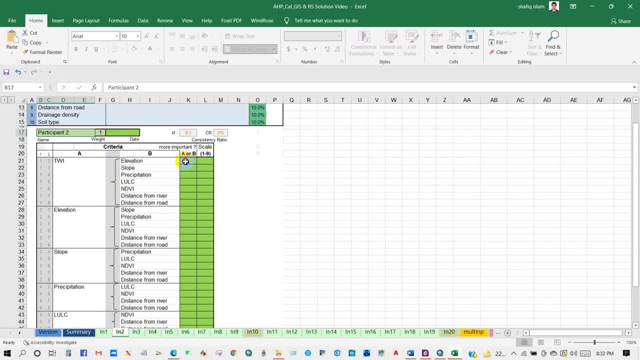 important, a or b. i mean twi important or elevation, i think a twi importance than elevation and it is a scale, one with equal importance. then twi or slope, of course twi and slope it is equal importance. then precipitation or twi a and both are equal importance. then twi or elevancy, it will be a. 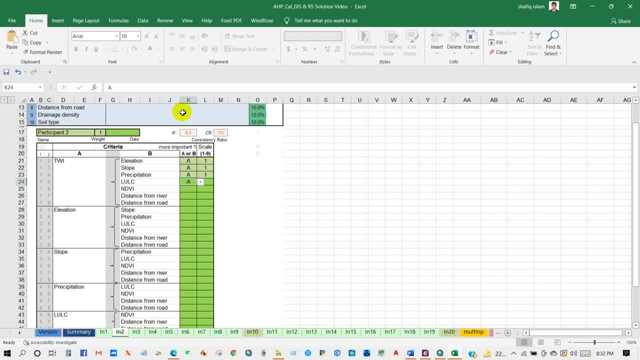 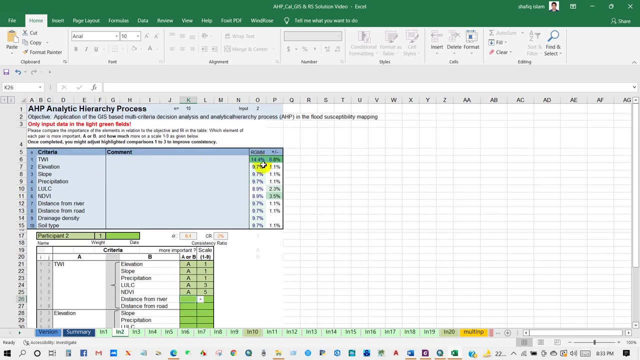 and then twi is important, then elevancy, so the scale will be three and twi and dvi. of course twi is more important than dvi, so it will be a, and in a scale it will be five and twi or and it will automatically calculate the weight here. 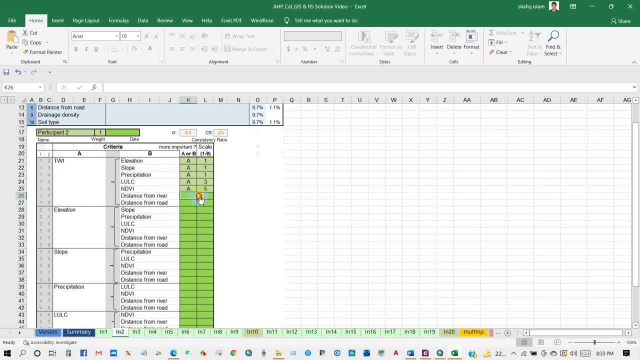 distance from river or topographic witness index, of course, topographic witness index, and it will be one, i mean equal, important, and distance from road, or twi, twi, and importance i mean in a scale, it will be five or three, or two, you can. it will be based on your expert opinion, the criteria and similarly. 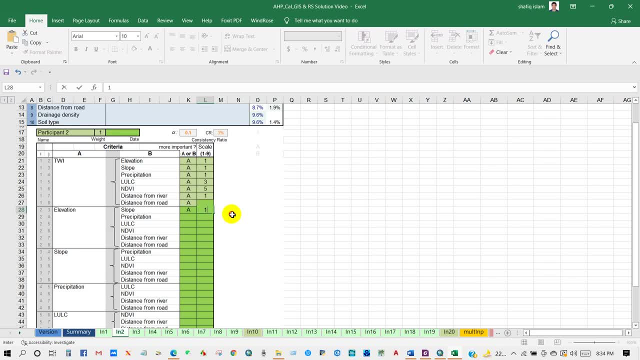 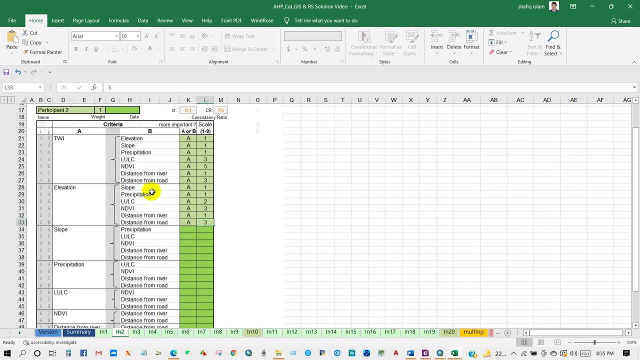 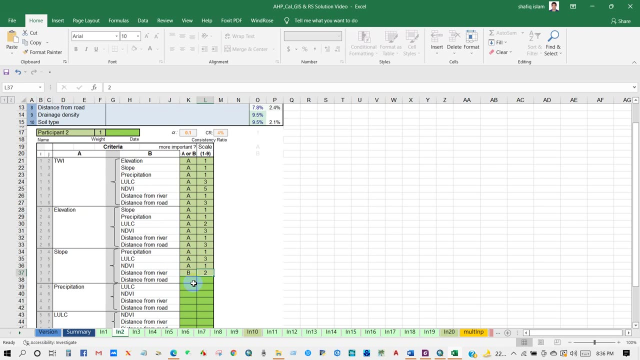 you can. it will be based on your expert opinion, the criteria and similarly you have to compare this criteria to criteria elevation or slope, elevation or precipitation, elevation, between elevation, lnc, elevation, ndvi, and put the scale, value and importance, like slope or distance from river. distance from river is more important than slope. that's why i write here b. 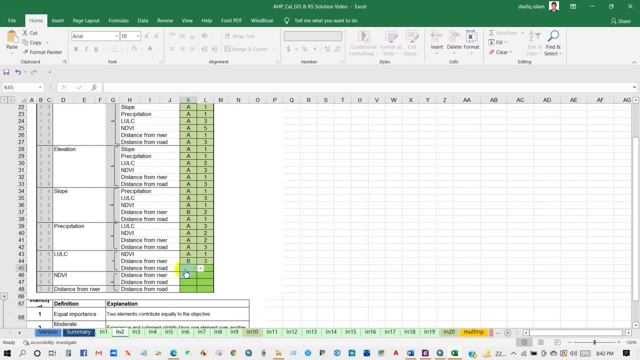 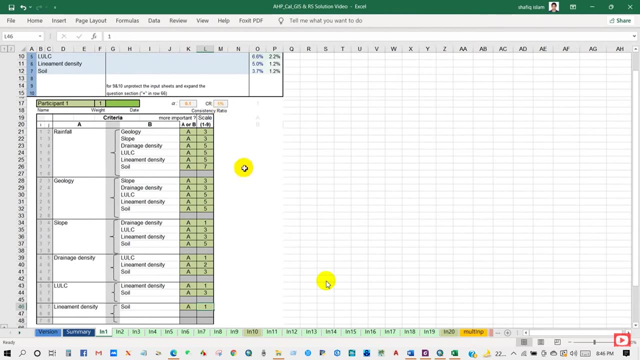 and here lllc or distance from river. distance from river shouldn't be the obscure version over river is more important than llc. that's why a and it is important in three scale. similarly, you have to write all the criteria here and for consistency ratio. for consistency ratio, you have to 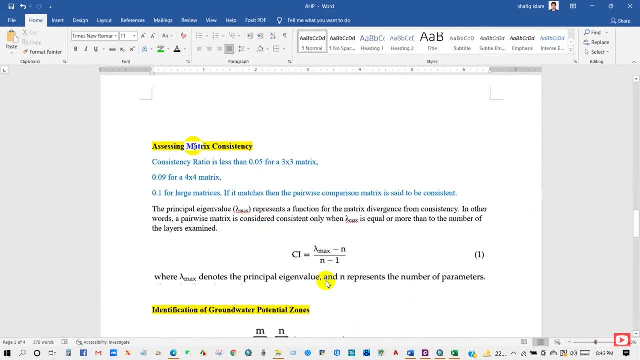 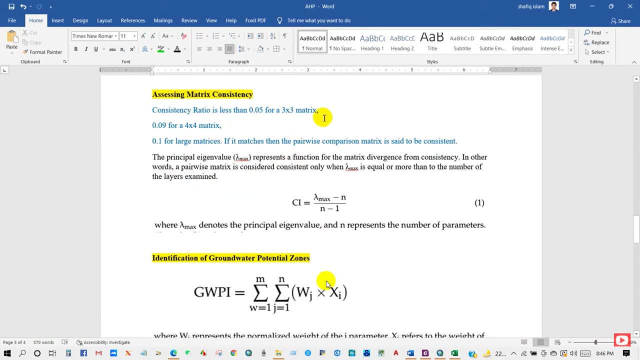 uh consider, ratio is less than 0.05 for 3 into 3 matrix and 0.09 for 4 into 4 matrix and 0.1 for large matrix. and if it masses then the pairwise comparison matrix is said to be consistent. 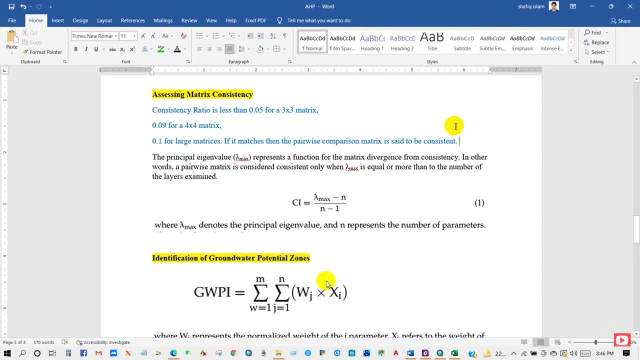 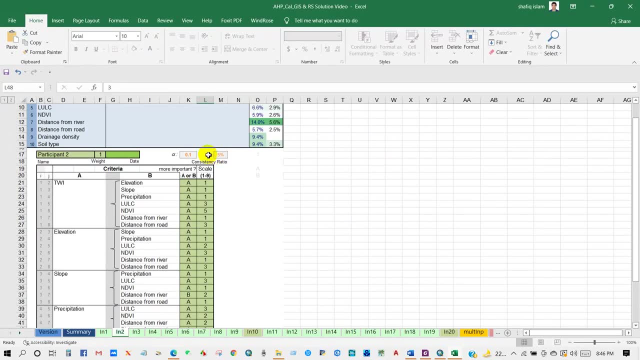 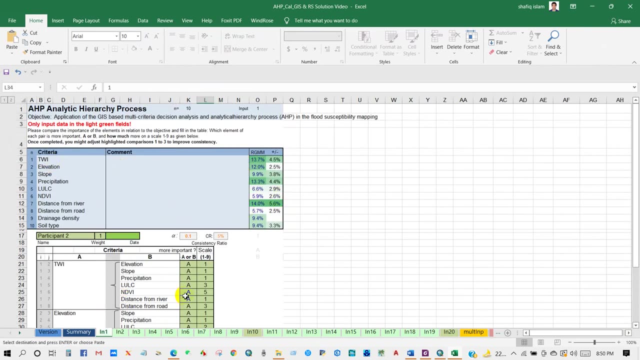 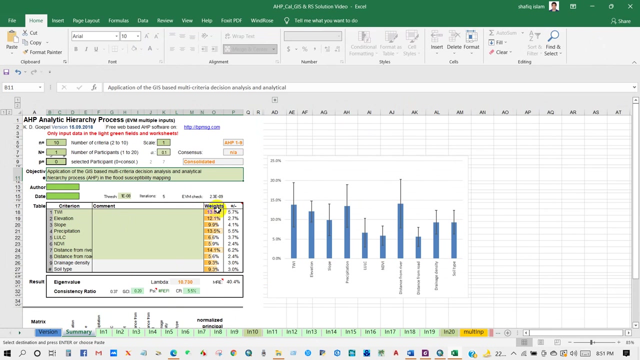 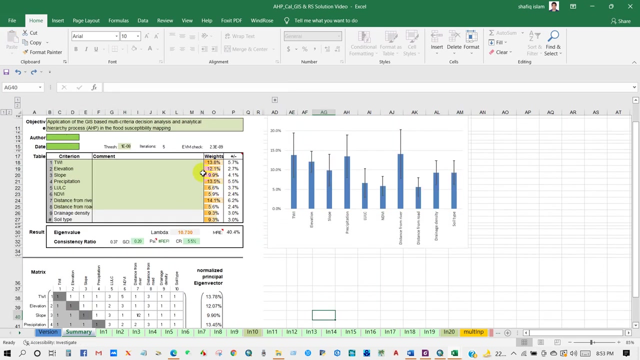 and it will be automatically calculated in the asp excel sheet. using this formula you can see: our concentration ratio is five percent, i mean 0.005, and the weight is automatically calculated here. finally, you can see here weights for all factors and here matrix and also normalized principal lagging factor. 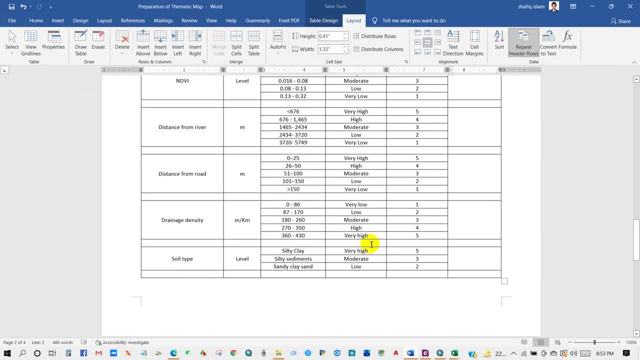 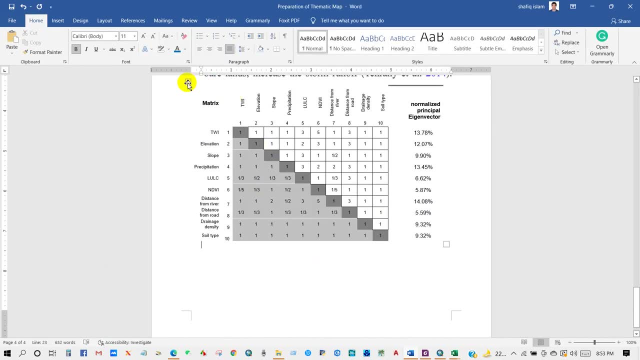 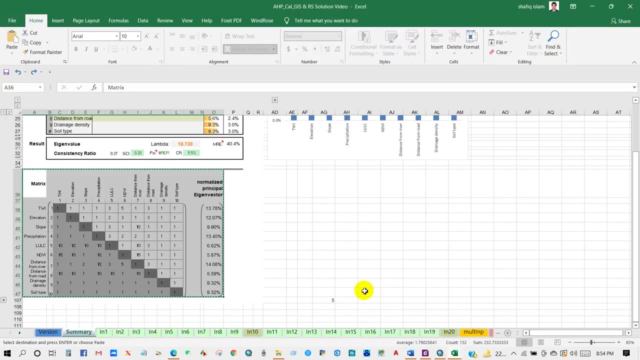 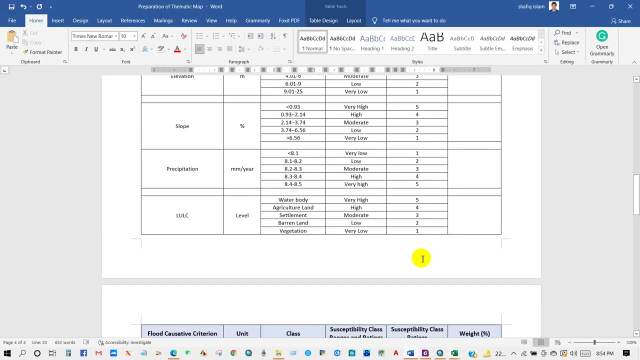 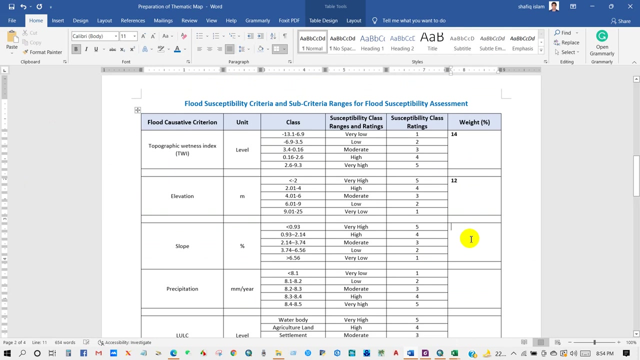 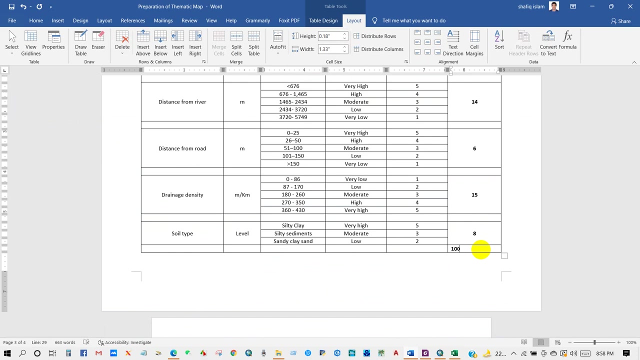 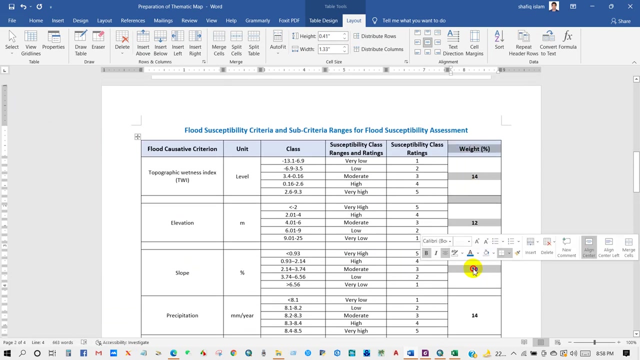 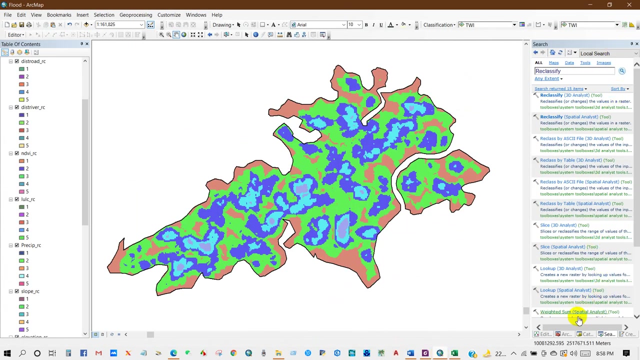 you can use this uh matrix in your study report. so now i will write here the weight for twa, it will be 14, 12 for slope, it will 10, and the sum of factor it weight, it will be 100. now in arcgis i will put all the factors and weight using uh overlay weighted technique. 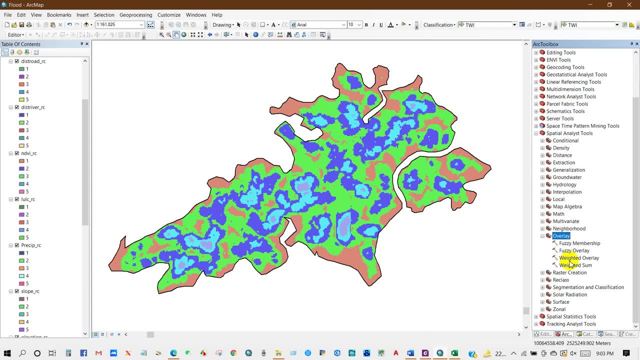 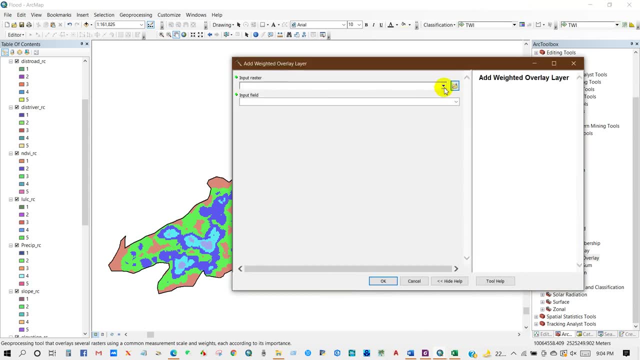 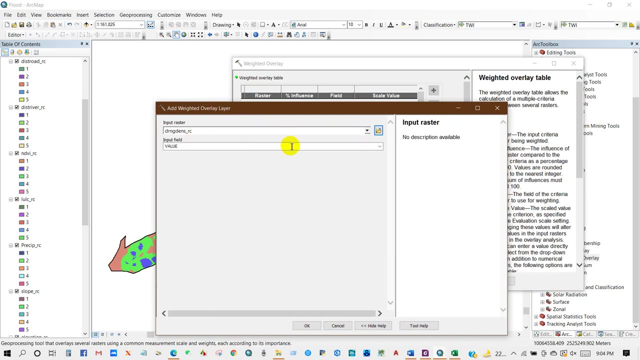 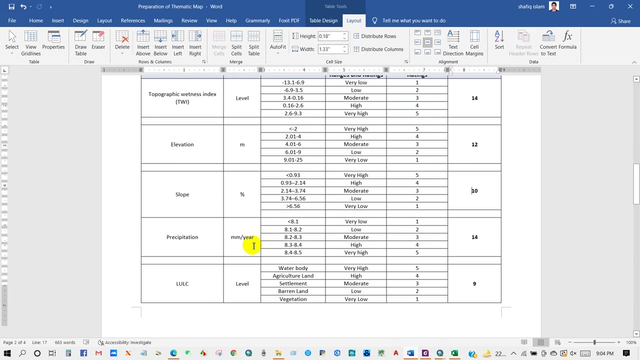 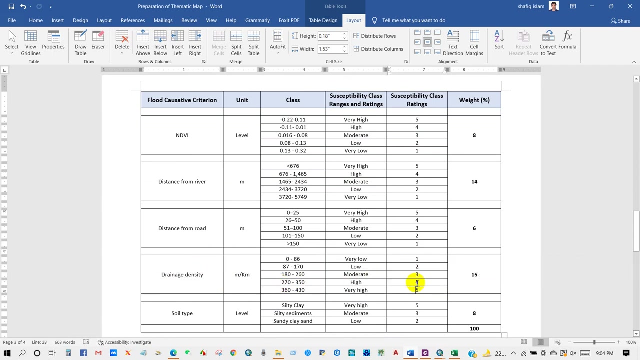 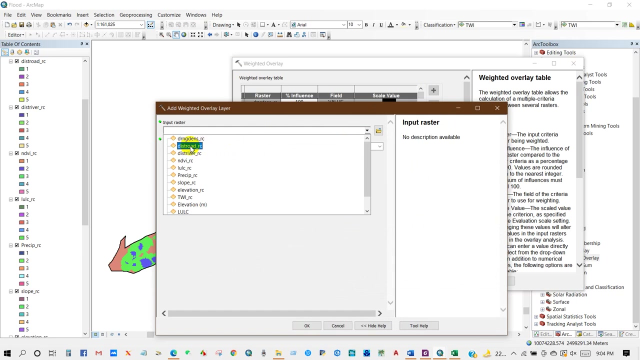 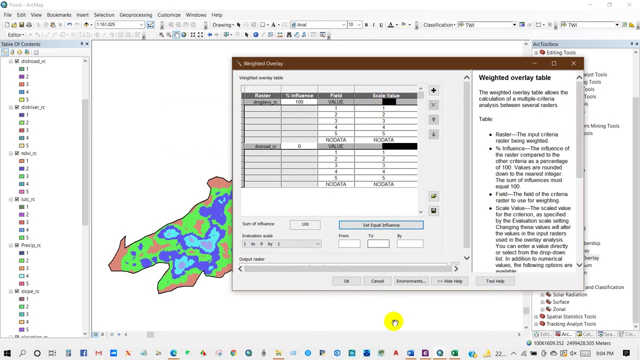 so for that go to overlay and then weighted overlay and add all reclassified factors. drainage density, then okay. similarly, add all the factors. and weight, then okay, add all the factors. here then is density, scale, scale value: add all the factors. distance from road: add all the factors: distance from road. 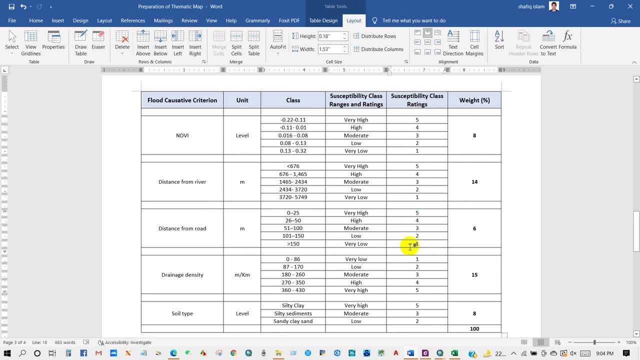 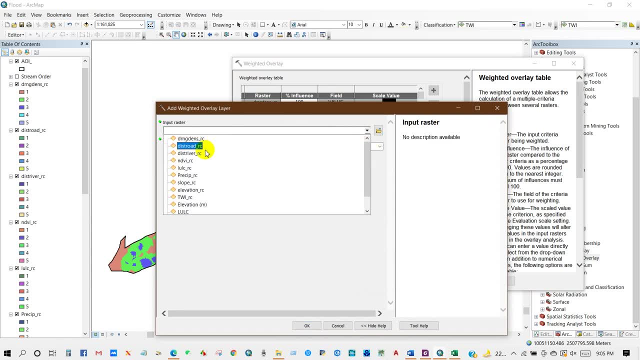 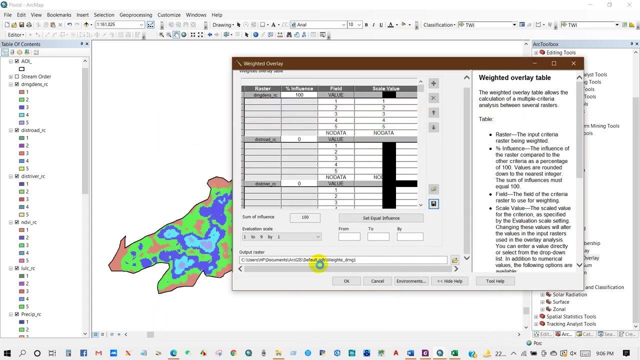 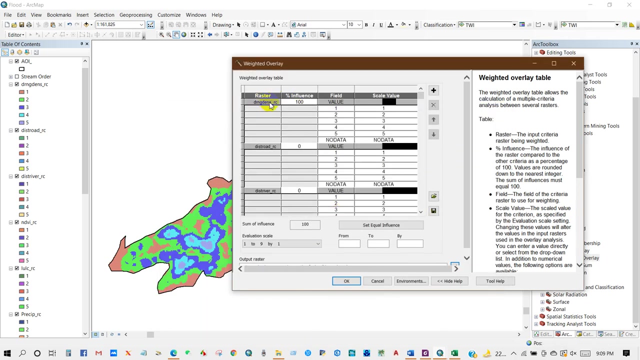 add all the factors: distance from road, distance from river, NDVI, LVLC. add all factors one by one: precipitation slope, elevation, DWI, topographic wetness index. after adding all the factors, you have to write the weight I. 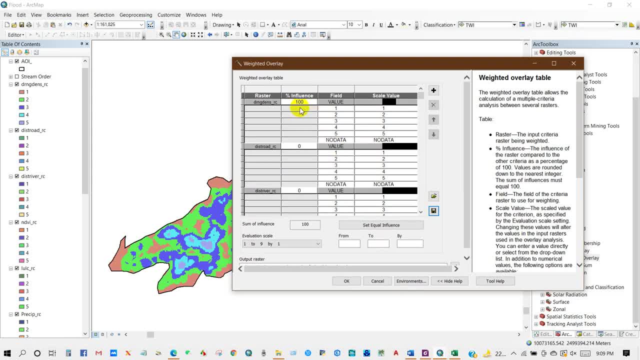 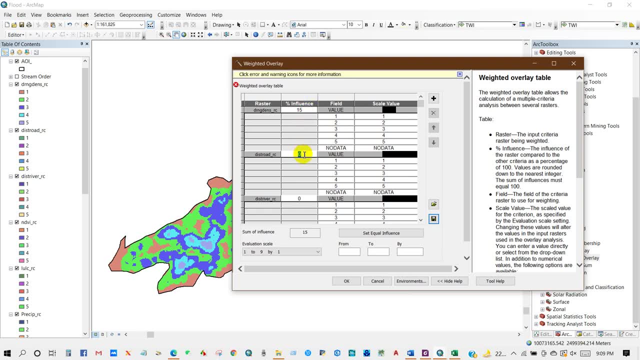 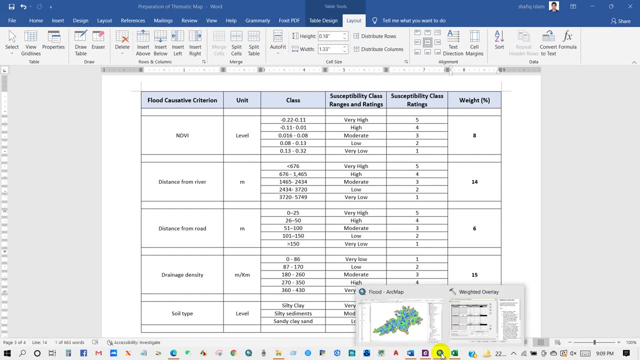 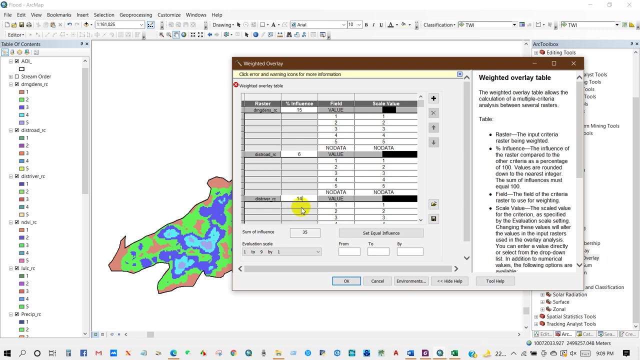 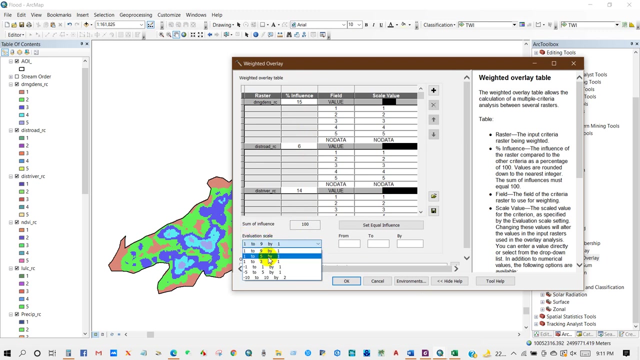 mean in full bands. here I'm here for drainage density. the influence is 15. I mean weight is 15, then distance from road, it is 6. similarly, you have to write here all the weights. it will be today. this is the potatis: 113, 16.